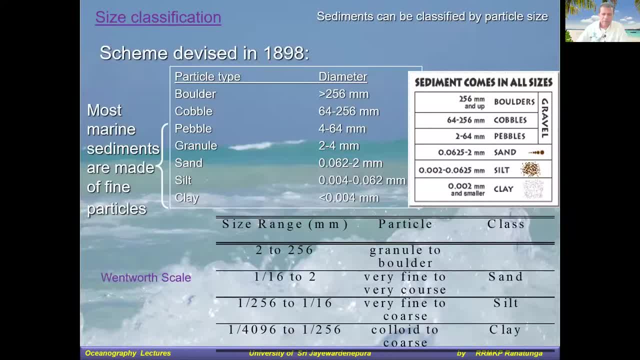 as well as they can be in different sizes. right a base on this, the size, you can name in different ways. in the simple terms: you know that's clay seals and you have heard about these things. but even beyond that, you can categorize sediments based on a more small standard. procedures like 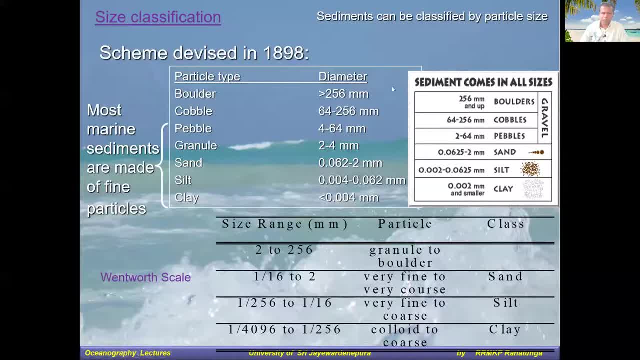 based on the diameter of the sediment. you can categorize sediments based on the diameter of the sediment, of these um sediments or even more scientific scale, like more different scales, like it's windward scale, where you can categorize sediments based on that scale, whether they are clay, silt, sand. 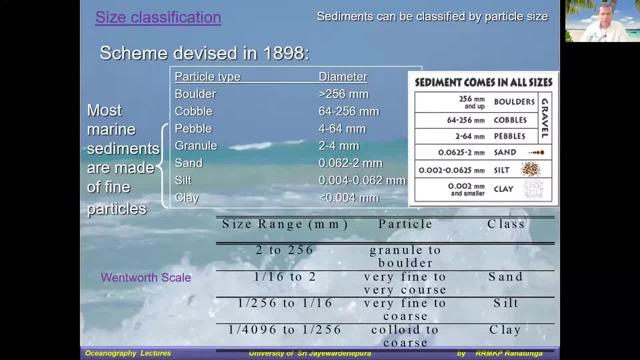 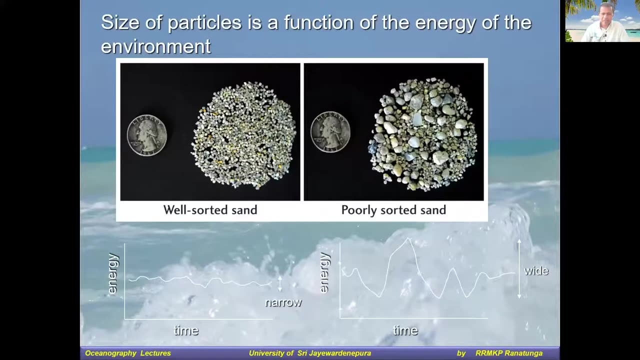 or whatever. there's boulders or like this. anyway, it just for your information only, don't try to memorize these things- and also the the size of the sediment i mentioned last week also. that is, it's an indication of the how much energy that these sediments receive. 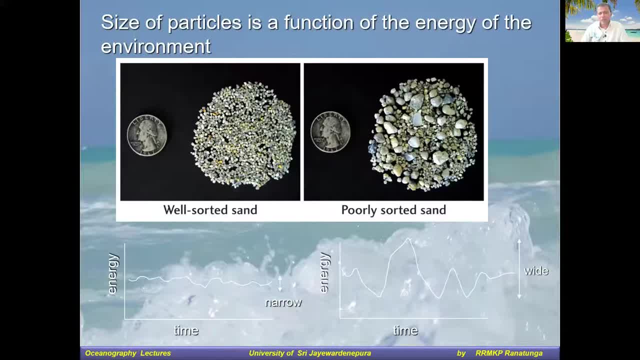 like, for example, if they are in the beach. if they are beach, sand like some sand may be larger, whereas the some of the beaches you will see very fine sand. so that again an indication of what kind of a the marine environment or how much energy or how much the wave energy. 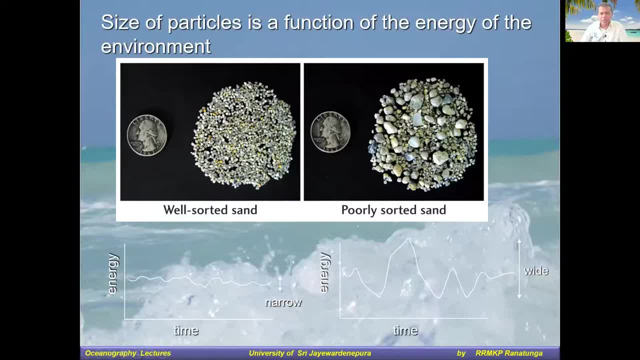 like, if it is a constant size range, sand particles, which means the, the waves are more or less equal, similar. but if they receive different types of waves in different times, then you will have different sizes in the in the beach. so next time when you visit a beach, you just see the size of the sediments in different places. you. 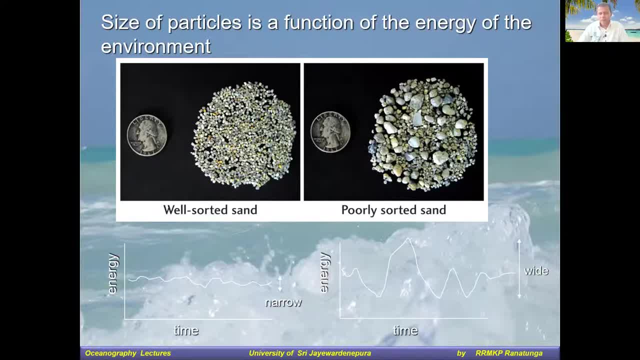 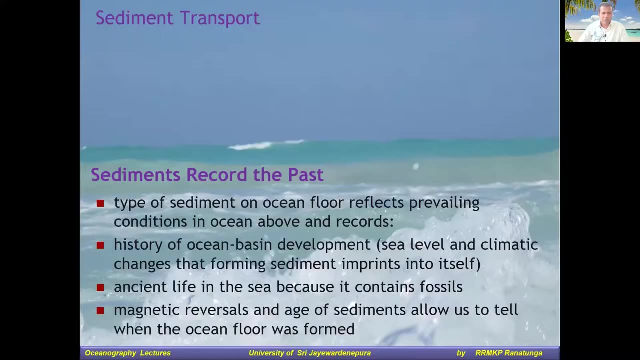 will notice they are different from time and place to play, so that can be an indication how strong the waves can be. so keep that one in your mind and observe this next time. right. and also, i mentioned last week that the sediment can be used to record the sediment or the. 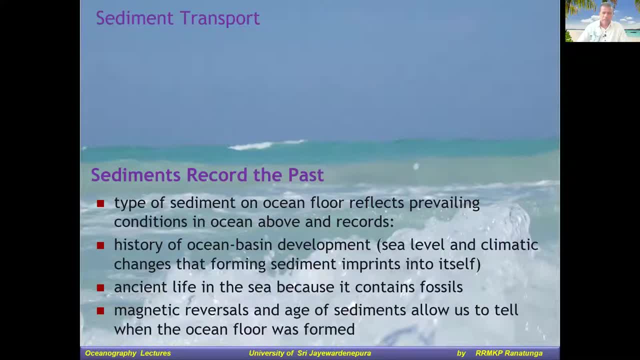 history of the earth or the sediment, because they are deposited layer by layer, year by year or decade by decade, or century by century, or sometimes even millions of years. they have been depositing the ocean bottom and that will give you some sort of the, the information for us to recreate or to understand what could have been. 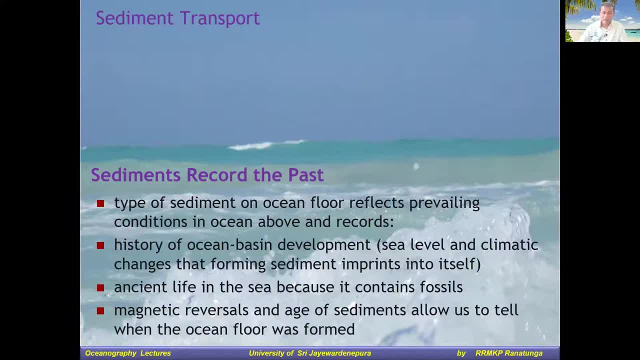 or how the earth could have been in the in the history, like different layers might have different animals or plant material trapped there, and they might have different trapped air bubbles where you can analyze how much the percentage of carbon dioxide, the oxygen the water column has collected by that time. so to do that one you have to get some what you call the 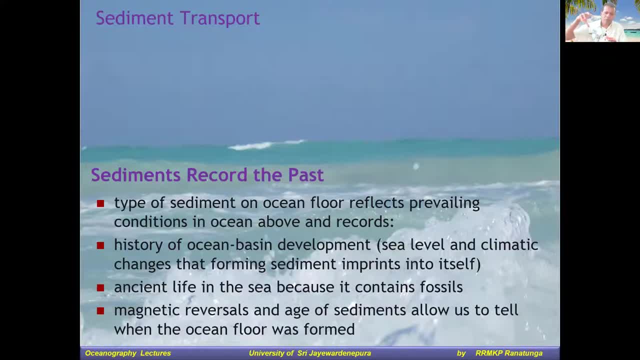 core samples. you send some sort of a sediment corer and you take the whole piece of rock or whatever the sediment material out and you do analysis, layer by layer, to see what is there, and then you can get a good idea about what kind of animals could have been there. 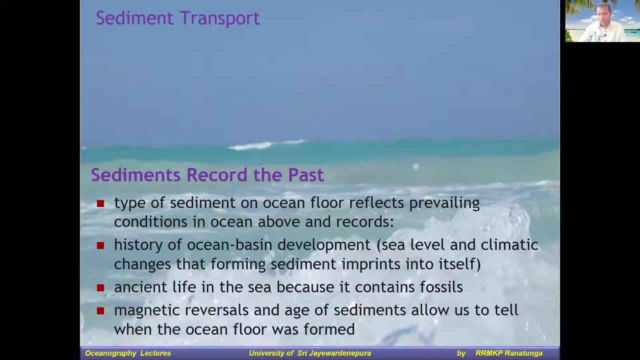 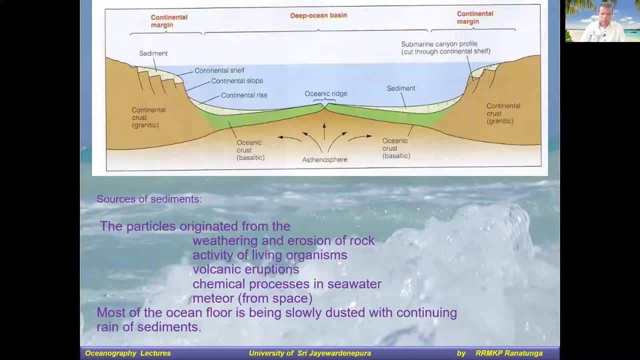 And you can, theoretically, you can- recreate how the world could have been in the history. That also very important for a scientist to work on. So, as we have already discussed and you know, these sediments are deposited mainly in the continental shelf, as well as in the continental rice. 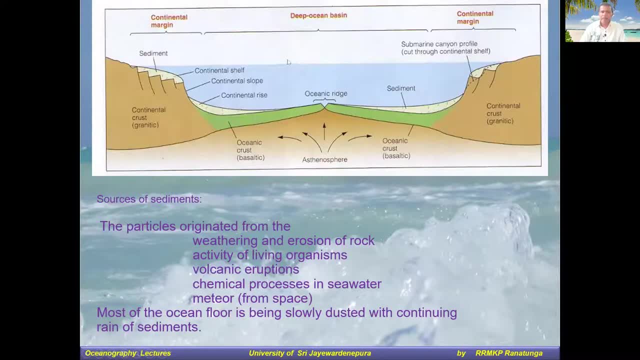 Mainly, but as by now you know that some of the sea flow is forming newly here We discussed last week that the sea flow spreading, or new sea flow, is formed from the mid-ocean ridges. That means they also giving some sediments. 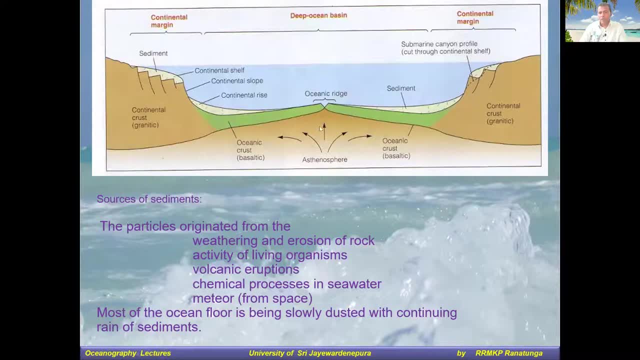 I mean this: when they, the material, come to the surface, they also some sort of a sediment. So they also added new sediment to the ocean bottom And the warm water or the hydrothermal winds. you remember that they also produce some sediments. 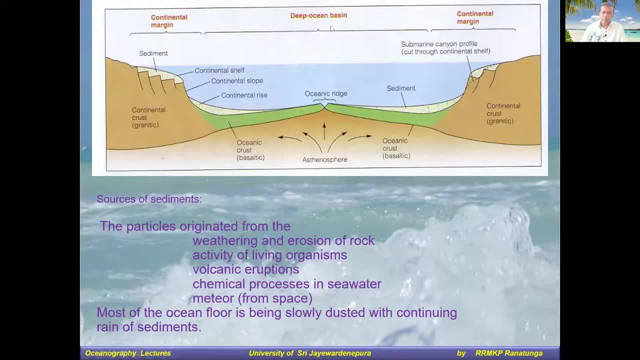 Other than that we get sediment from the, even from the outer space. So, And these are the, the, the, basically where the, the ocean gets sediment from, That's the weathering of erosion, weathering or erosion of rocks. 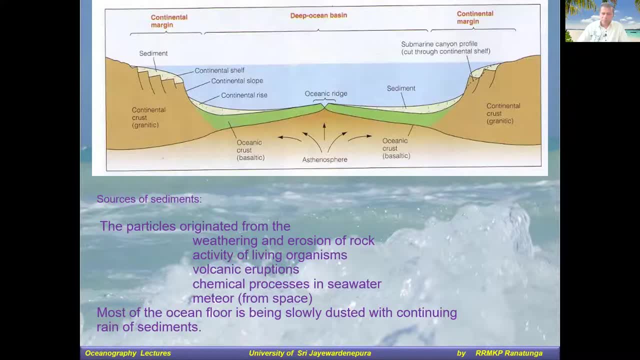 And then pass on uh to your name. so I got the name uh, giving a cracker thing. you know they need you in the cracker thing. the summer sediments have you know. uh, no, guinea can. 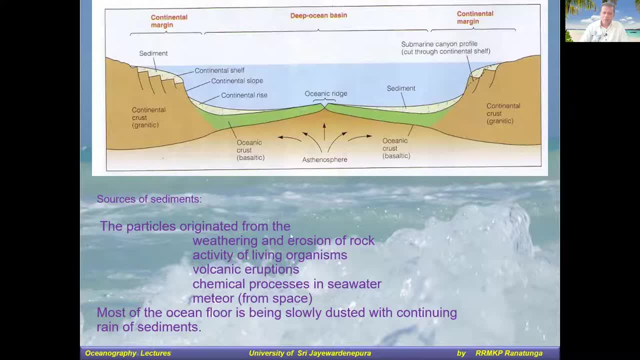 do people in volcanic eruptions, And then We're going to talk about the Mulan centre, because Tyalur and the very last ever, uh, uh, uh, uh, uh, uh, uh, and then and then it was like you know. 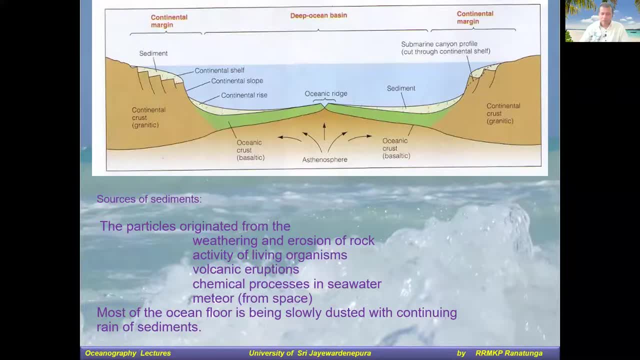 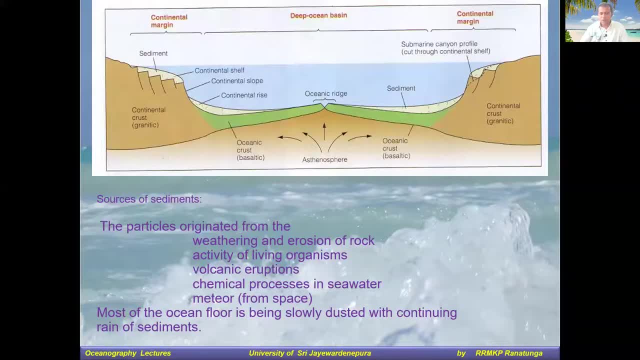 Casio carbonate. It's put to one more statement. So, uh, We can make natural salt from this soil. This is what is called as Euperites in geology. This is what is called as Euperites in geology. 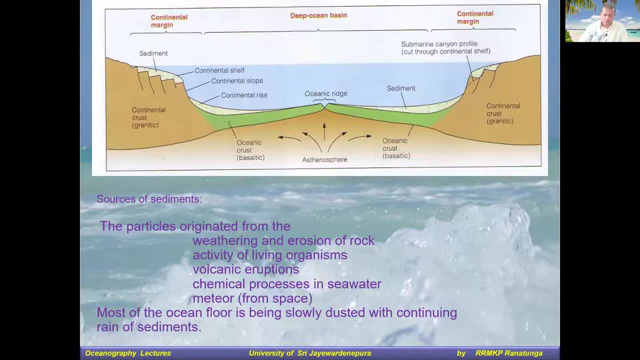 It is just salt. Especially, salinity is very high. It is found in the Arabian Sea, Jordan and other places. It is found in these rocks. It is found in these rocks. There is also a sediment group. There is also a sediment group. 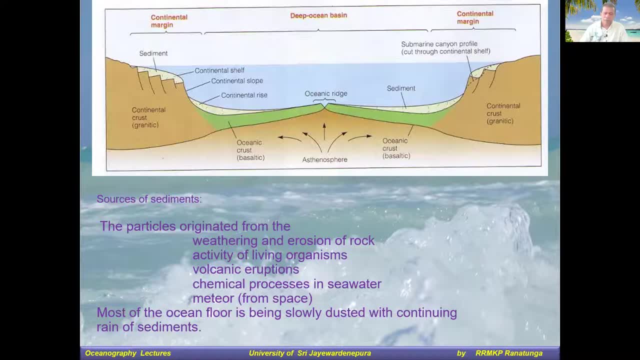 We can use it for the soil. We can use it for the soil. It is not easy for us to make such a product in Sri Lanka, because we do not have enough resources. Also, if the weather is bad, we may not be able to get these sediments in the future. 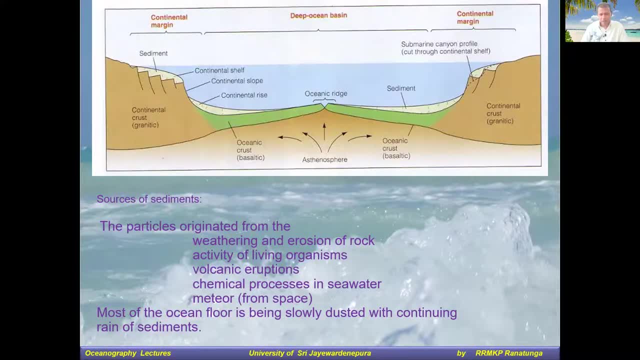 This is not a big problem, but the sediments that are used in one of these processes are in this period, But the weather is bad, so these sediments are constantly being stored. in these sediments. Sediments are stored in large quantities. 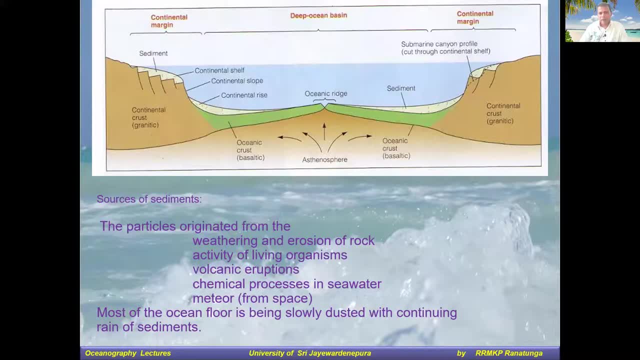 So these sediments are getting better in various ways. Some sediments are called minerals. Some sediments are stored in large quantities. Some sediments are called oil and gas. Oil and gas is a very big product. It is said that it is made in a medium quantity, but it is not made in a new way. 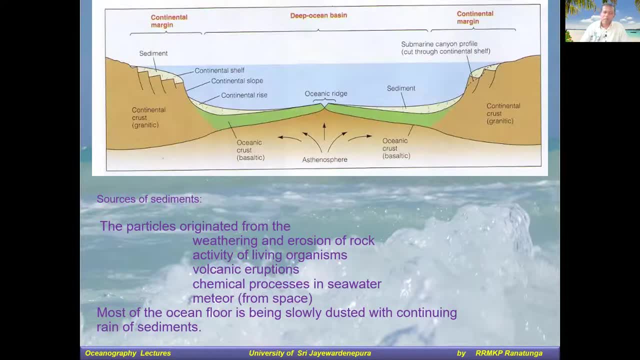 It can be made in a medium quantity. It can be made in a medium quantity. It will be matured. It will be matured And it will be aged, which will also make another AUDE. Likewise, there are many uses of sediments as well. 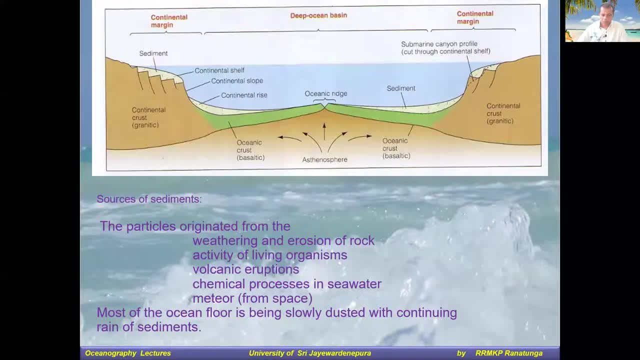 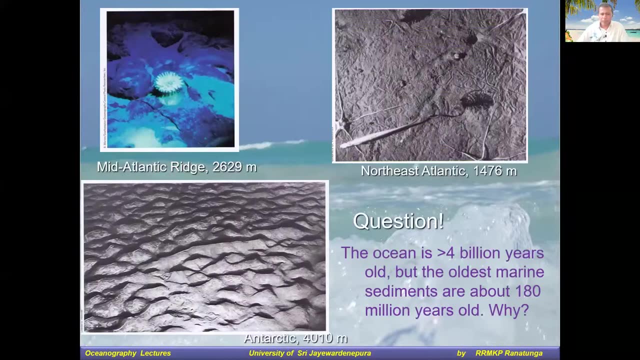 We will discuss towards the end. when we are talking about the ocean uses, For example, when we talk about opportunities like farming and goods are obtained, We see effects of these in the OSCE Stat Department, which are in low pressure, Pintura, Mid-Atlantic Ridge, Mid-Ocean Ridge and so on. 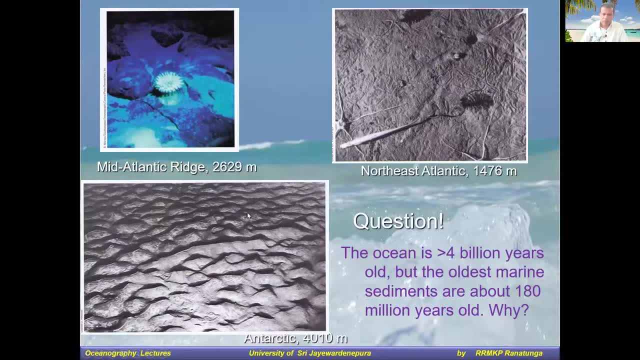 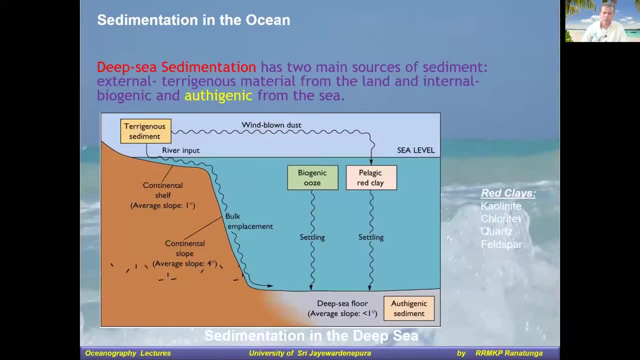 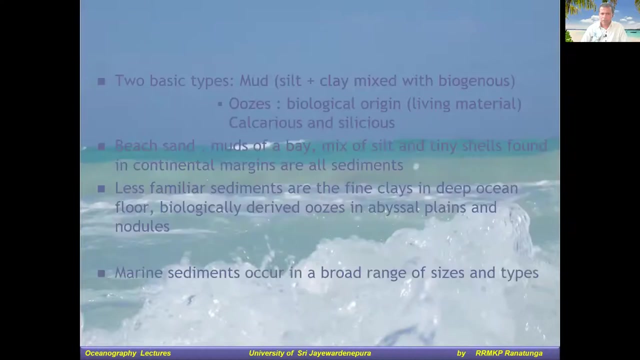 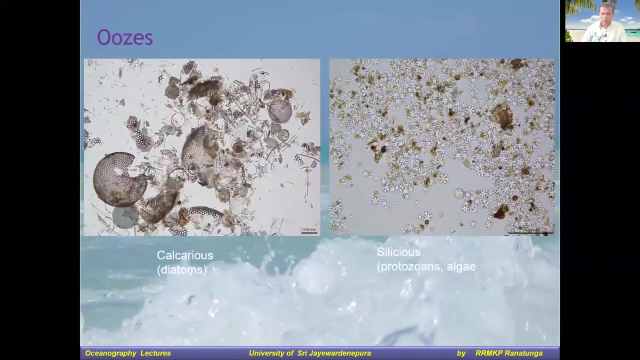 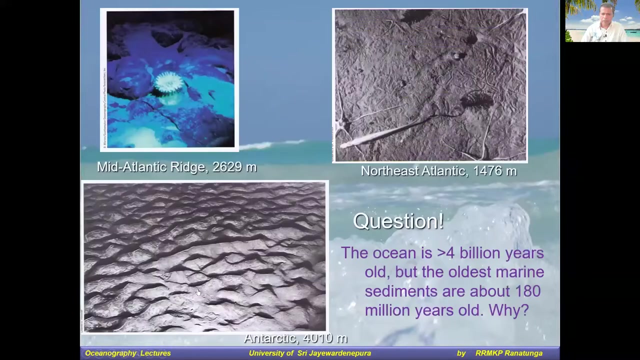 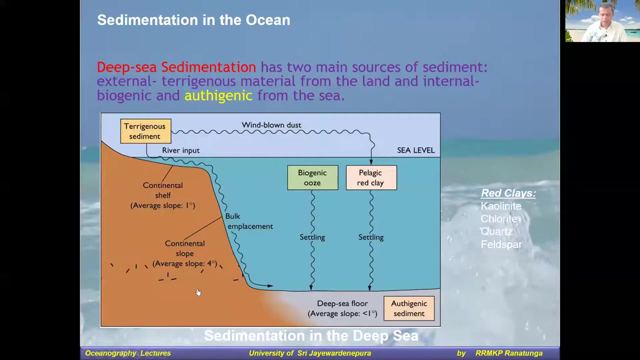 So that's where actually we stopped last week. And one thing I forgot to mention: that the classification of this sediment- actually the very beginning- should be next to this one. Basically we divided the sediment into four groups, But in some of the publications they're talking about the five types of sediment. 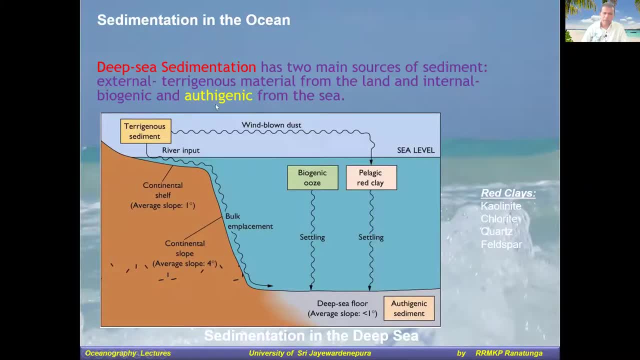 For example, in some documents there is something called orthogenic sediment, which refers to something naturally, or some sediments that form naturally in the marine environment. Orthogenic means naturally, But it has no scientific base. Usually we talk about the four different types of sediments: the heterogeneous, the biogenic, the cosmogenic. 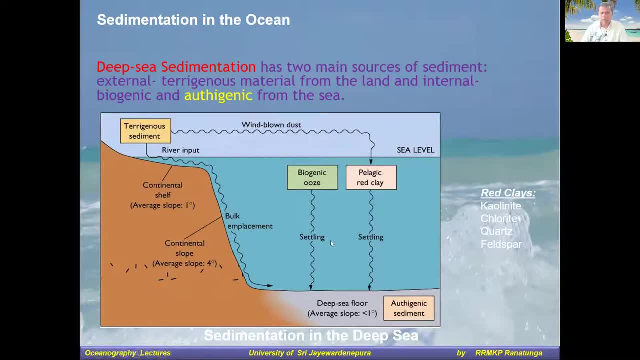 Hydrogen is sediments which we will come to Like. in this diagram you will see where the ocean, especially the deep ocean, get this sediment from The terigenous sediments. if you remember, last week, I think, I mentioned: 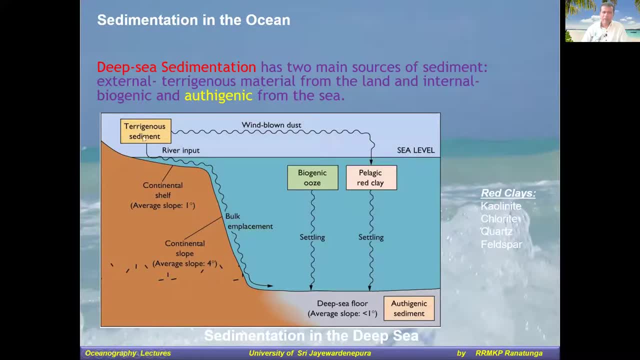 the terigenous means, the sediment that formed from the rocks, Whether they are weathering or erosion of rocks. that sediment get into the sea, mainly from the river inputs, when they are deposited in the continental shelf, or even beyond that, to the sediment, the turbidity currents. 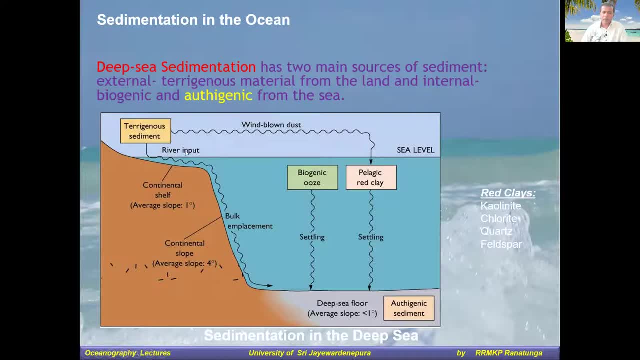 I hope you remember now the sediment here. They can flow to the ocean bottom as the turbidity currents And they are deposited here. So all these are terigenous sediments And the others are the biogenic sediments that due to the activities of the organisms 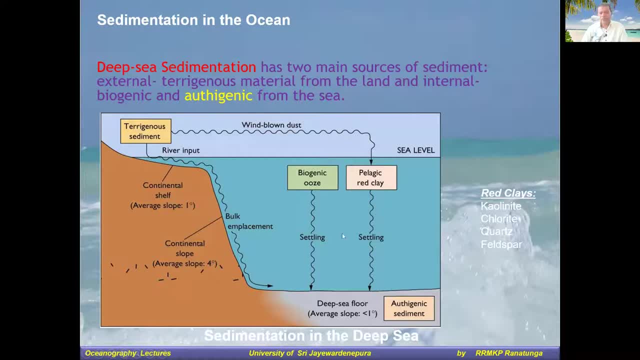 the biological activities of the organisms. there can be some sediment form in the water column and they can be settled. So actually these biogenic sediments, or sometimes we call the biogenic oozes they are once they are settled in large quantities somewhere here. 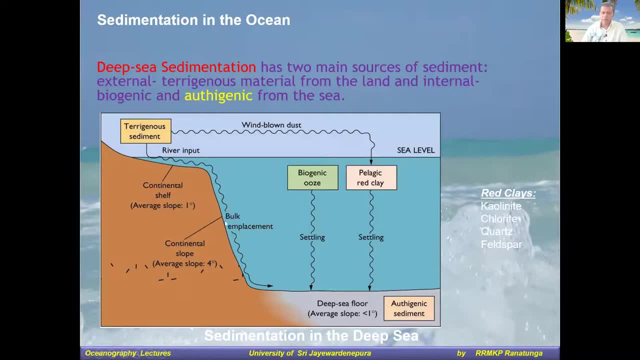 and they are covered with the other type of sediment, especially from the terigenous sediments. layer by layer It can be sometimes hundreds to meters to several kilometers deep sediment would be deposited on top of that biogenic sediments And that is actually the source of the oil and gas. 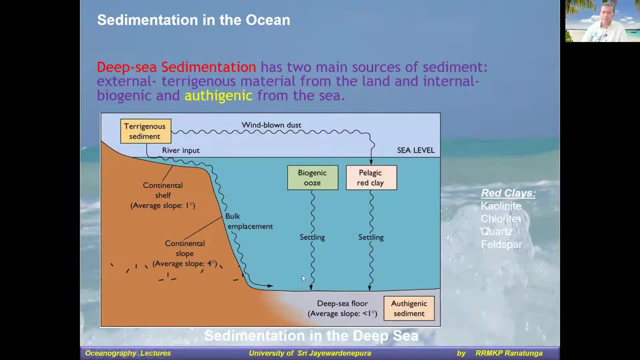 These the biogenic sediments. when they are deposited- and they are under very high pressure because of the water column above as well as the other sediment layers- they will be in a very high pressure as well as in the high temperatures In that particular temperature. 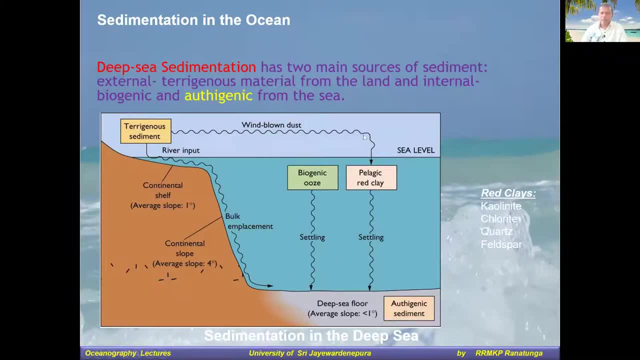 and the pressure they start forming this oil and gas. It depends on what temperature and what pressure they are and decide whether they are going to be natural gas or whether it's going to be a what kind of type of a crude oil. 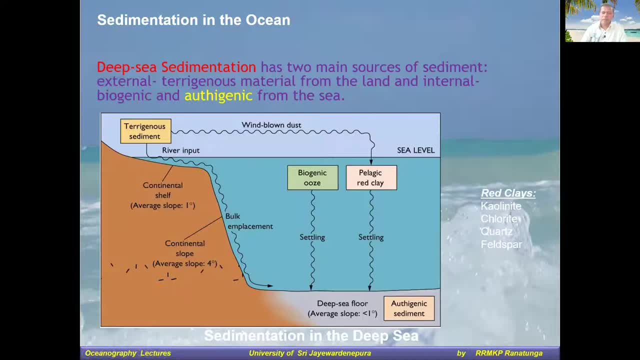 We call it Bortel, In that Bortel work the natural gas that they use to make the sediments after that pressure, and then after that it will melt. It will melt when it comes out of the water. In that case, 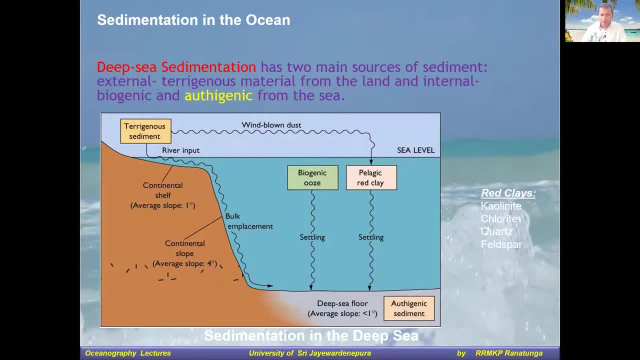 these biogenic sediments, otherwise later on these natural gas or oil and gas, etc. So the same terigenous sediments, they can be come from the river, but also they can come as the blown dust that comes out of the water. 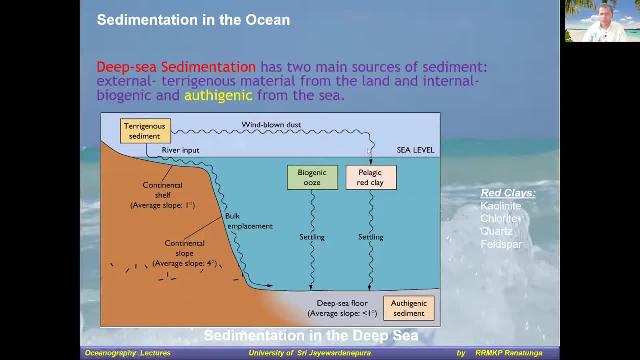 and they can also come out of the mud. If you are a person like me, I don't know. but, for example, I have a story about this, Veli Kunatu. I don't remember where it came from. I don't remember. 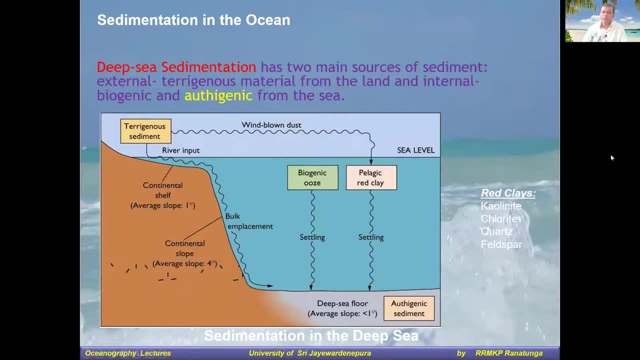 In addition to that, the Veli Kunatu, like the mud, can also come out of the other continents. like the mud. For example, if you go to a very powerful pond like this, like this, it will come out of the mud. 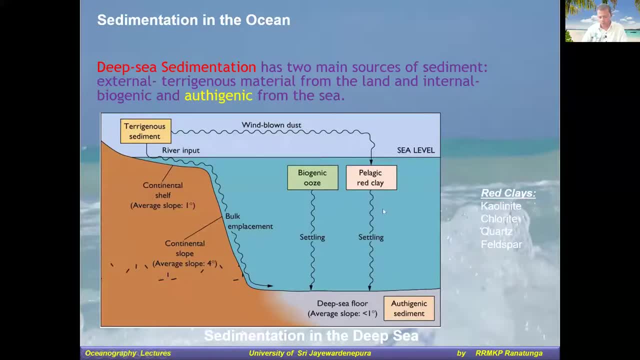 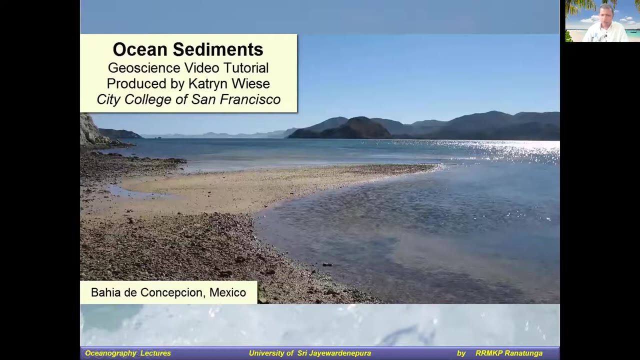 and they deposit it and it will settle there. That way, if you go there, the sediment deposit will be there and at the end they become marine sediments in general, right, So let's see little bit further on the marine sediments. 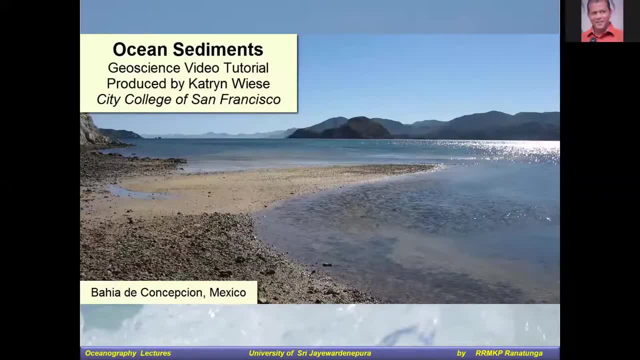 I have a small video clip. we can watch that one and we'll come back. In this video, we will look closely at the sediment that makes the top layer of ocean crust. Where does it come from? What does it look like, Feel like? 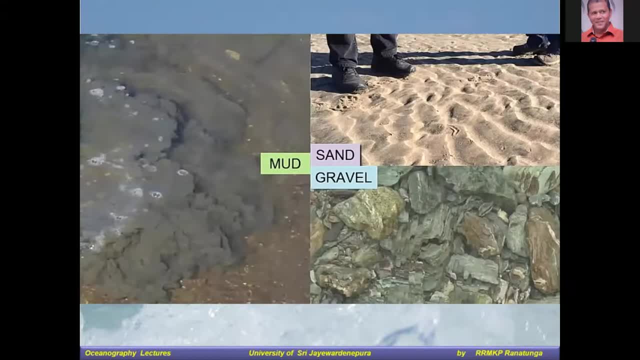 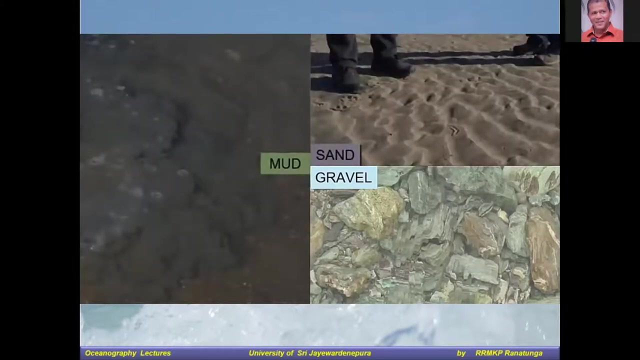 Let's start with the vocabulary used to describe sediment size. There are many terms used to describe sediments of all sizes. We'll simplify them for this class into three categories: muds, sands and gravels. Technically, gravels are sediment grains larger than 2 millimeters in diameter. 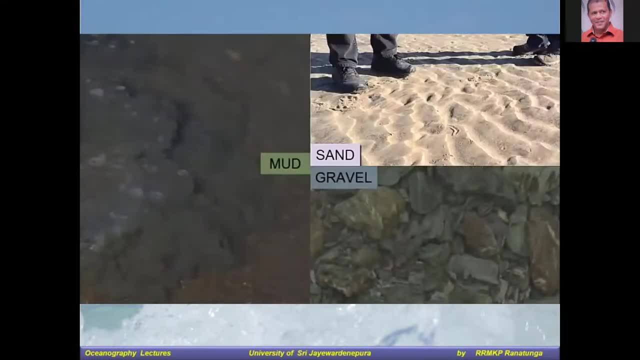 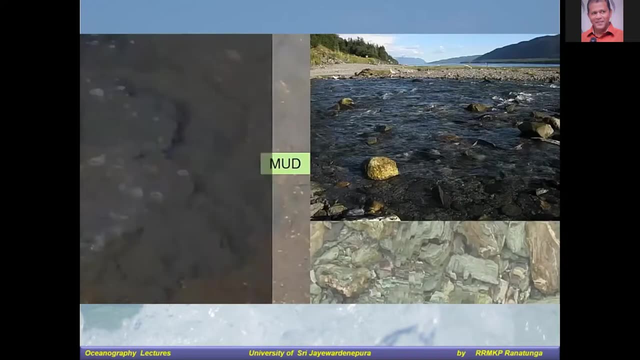 Muds are less than 1 16th millimeter. Sands are everything in between. Where is each of these grain sizes found? in the ocean? The largest grains, the heaviest, settle quickly in still water and require high energy water to be picked up and carried. 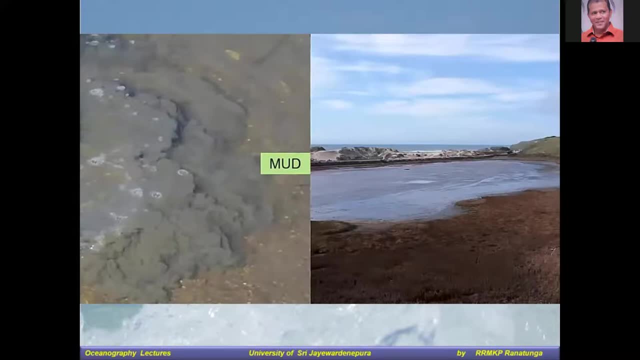 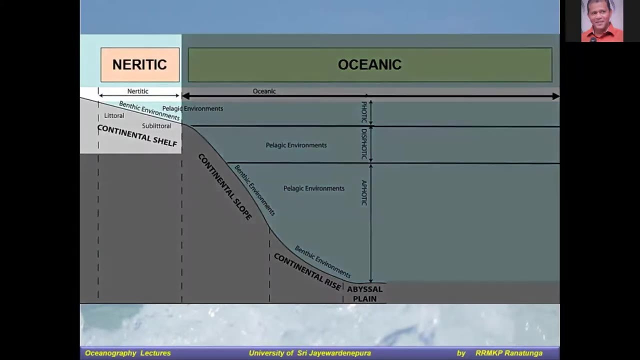 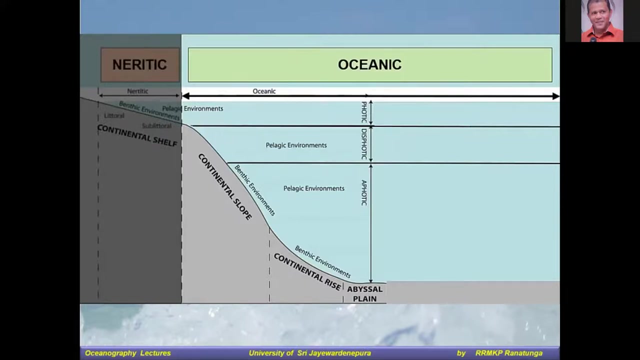 The smallest grains require perfectly still unmoving water to settle out. Ocean environments are separated into two major geographic zones: Neuritic over the continental shelf and oceanic over the slope rise, abyssal plains, mid-ocean ridges and trenches. 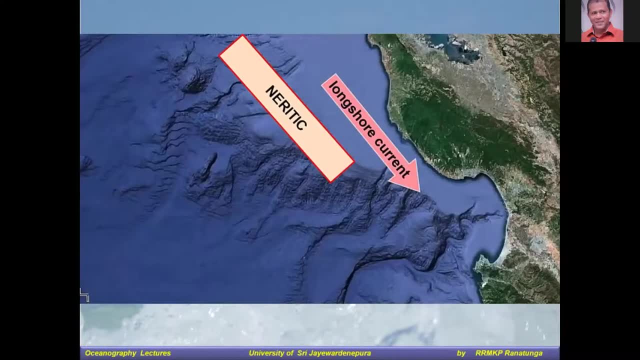 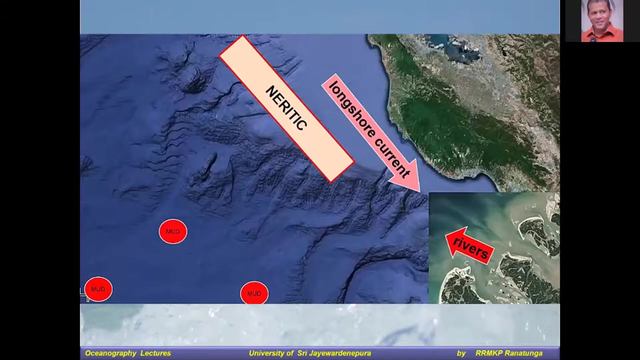 Neuritic waters tend to have faster moving currents interacting with surface waters. in the shallow bottom, These waters can pick up and shift around larger sediment grains. Rivers that enter here will retain mud-sized sediments in suspension and can carry them quite a distance offshore. 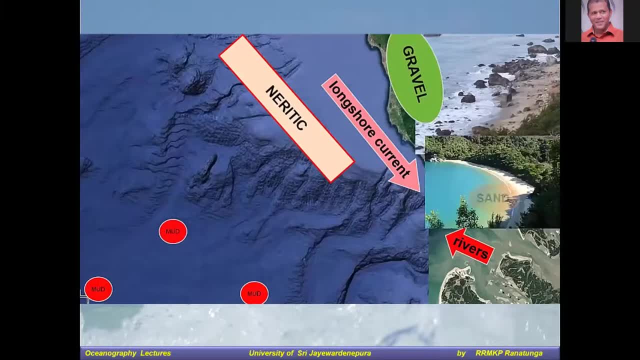 Gravels tend to stick close to shore. Fine sands collect in medium-energy coves and can be carried out to the edge of the shelf. Muds settle out only in closed-off, no-energy lagoons. Oceanic waters are deep with no currents that touch the bottom. 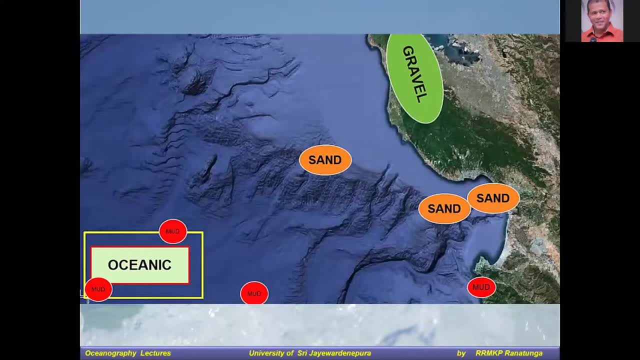 Gravels and sands cannot be transported out here by anything other than floating icebergs, So the sediment that falls here is only the suspended muds. Where do these muds come from that get out to the oceanic zone? Nearby rivers that have a lot of suspended sediment. 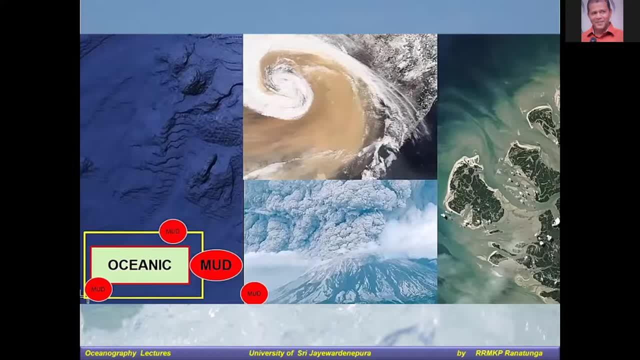 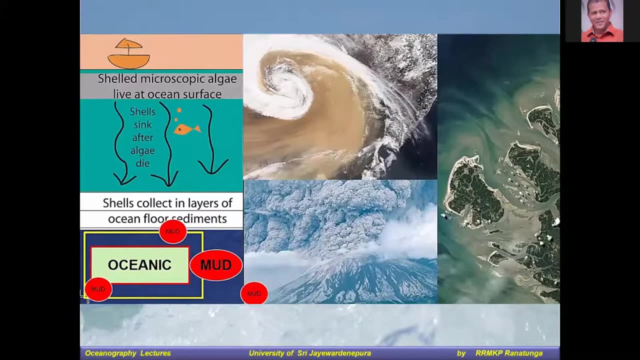 Airborne dust and ash that settles on the surface, And the shells and debris of organisms that live in the surface waters and settle to the seafloor when they are in the ocean, And then those organisms die. The oceanic zone represents four-fifths of the world's ocean environments. 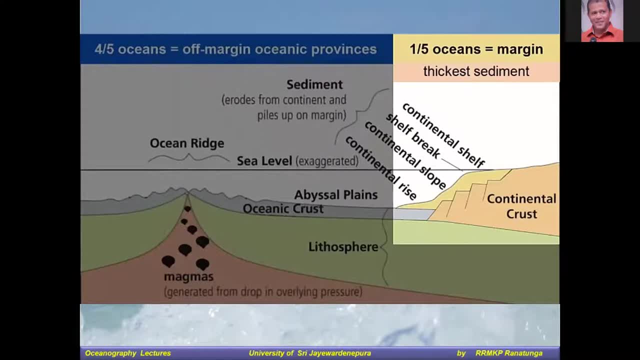 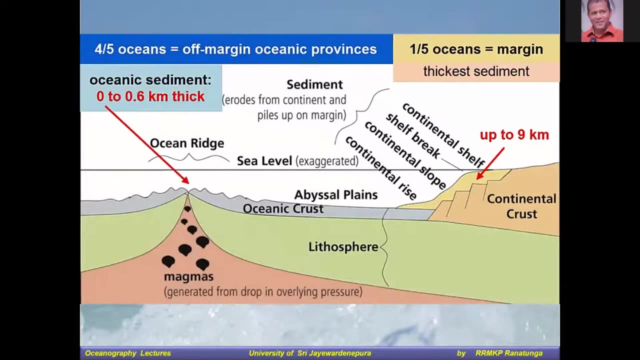 However, the sediment that collects in the margin environment is the thickest in the world, up to nine kilometers thick compared with the oceanic sediment thickness, which increases from zero at the ridges to 0.6 kilometers at the thickest oldest edges of the abyssal plains. 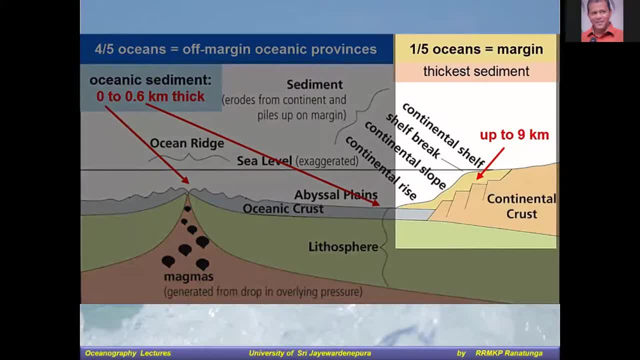 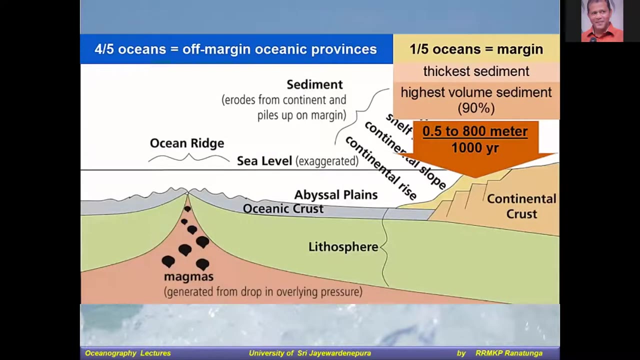 Even though the sediment that collects in the margin environment represents only one-fifth of the ocean's surface, its sediment volume represents almost 90% of the total ocean sediment. Why Sediment collects here much faster, at rates from a half to 800 meters per 1,000 years. 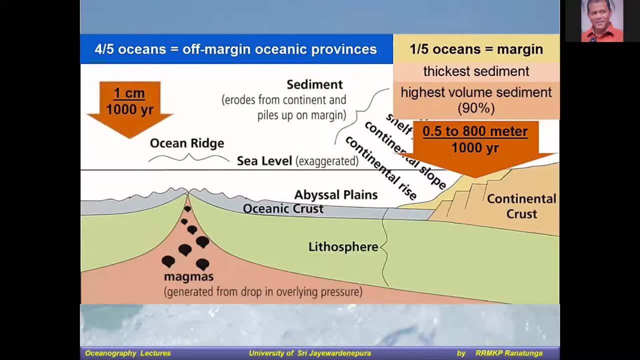 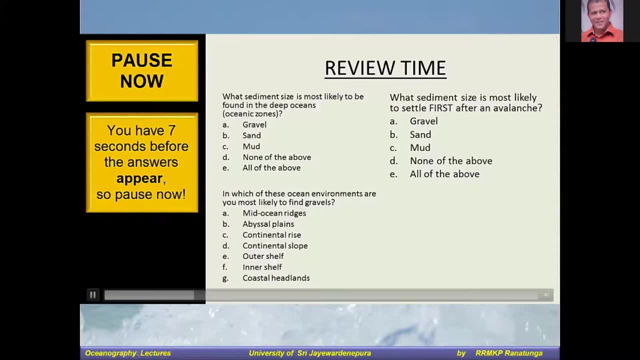 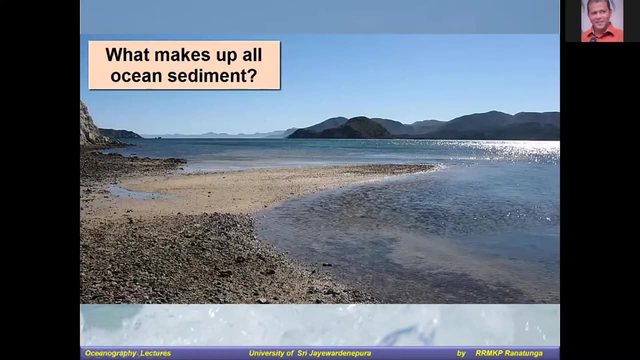 For comparison, in the oceanic zone, sediment collects at its fastest: 1 centimeter per 1,000 years Pause. now, What makes up all these sediments? There are four major sources of sediment to the ocean, and of course each gets its own name. 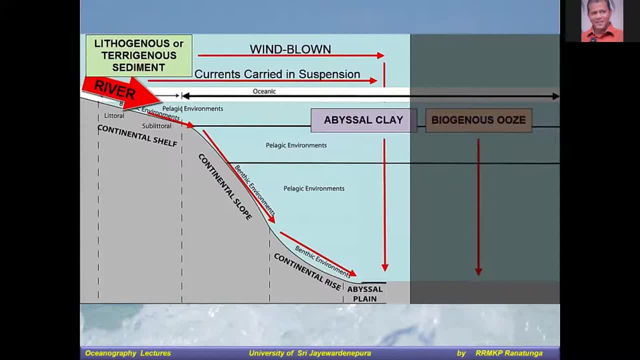 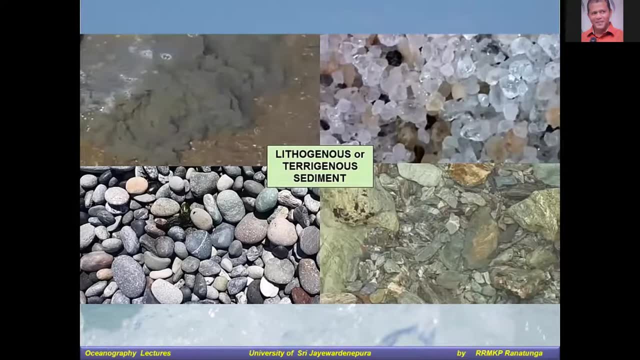 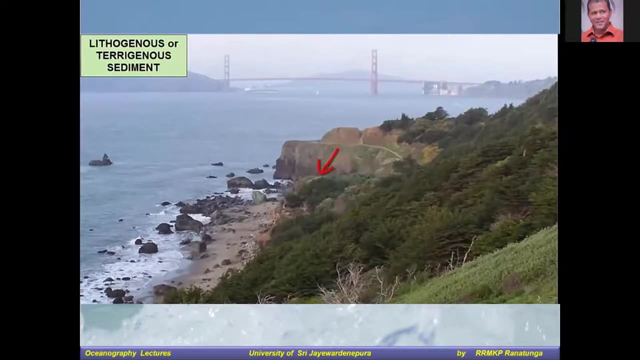 We call sediment that originated from rock weathering on land lithogenous or pterygianus sediment. What is it made? of? Bits of rocks and minerals. When, next to a weathering cliff, like along an eroding coastline, the material is made of bits of the rock in the cliff? 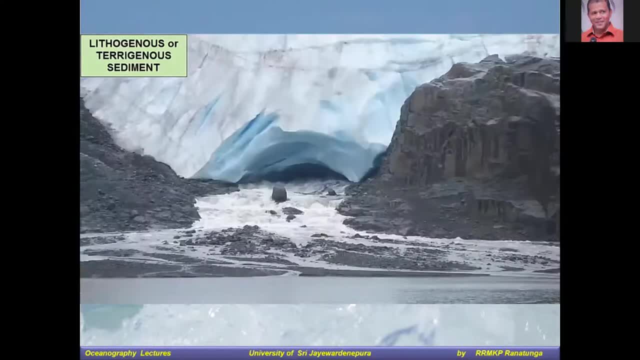 and gravity carries them towards the ocean. When dropped by glaciers, these sediments can be quite large and come relatively preserved from the backcountry far inland. We call both of these types of sediments immature because they haven't been modified much by travel. 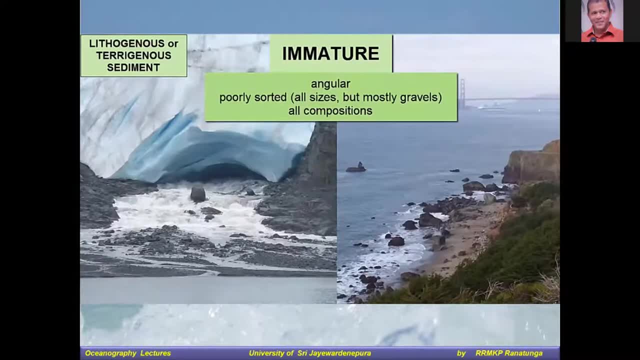 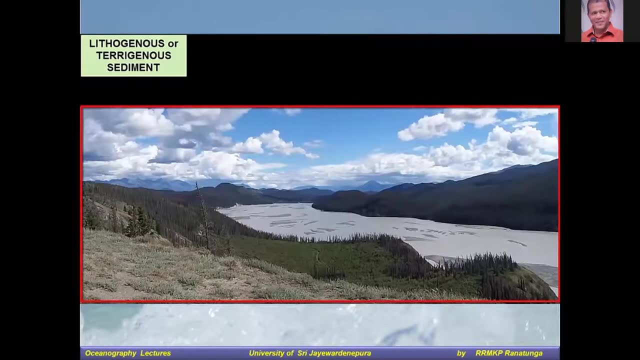 They can be angular and poorly sorted, consisting of grains of all compositions, shapes and sizes, mostly gravels. When lithogenous sediment is carried by rivers, on the other hand, it becomes mature Grains, decrease in size to fine sands and muds. 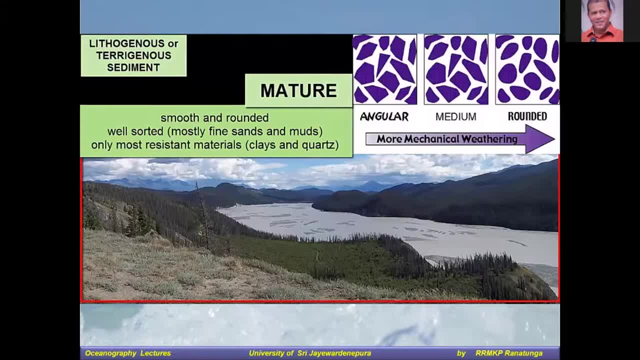 Why, During transit, the grains are knocked around and hit each other. They physically break down into smaller pieces. They also break down chemically. Most of the material dissolves or is turned into clays and rust. The most resistant materials: predominantly quartz grains. 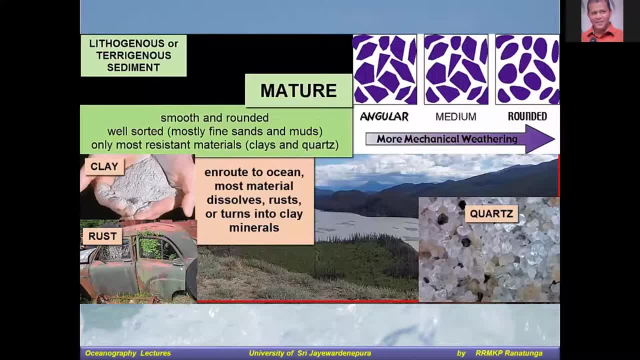 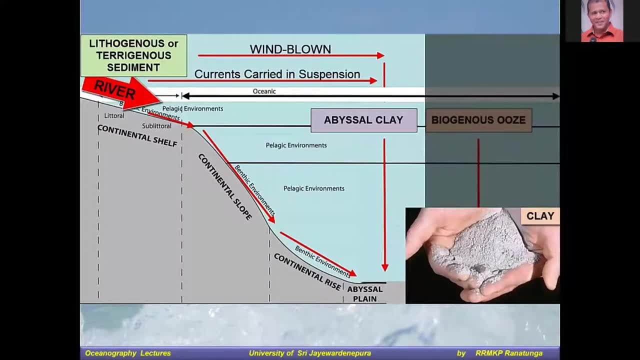 which don't dissolve or turn into clay or rust remain. Clay minerals are mud-sized and are the most common byproducts of rock weathering on Earth's surface. Some of these clay minerals make it out to the oceanic zones, either by being held in suspension near large river deltas. 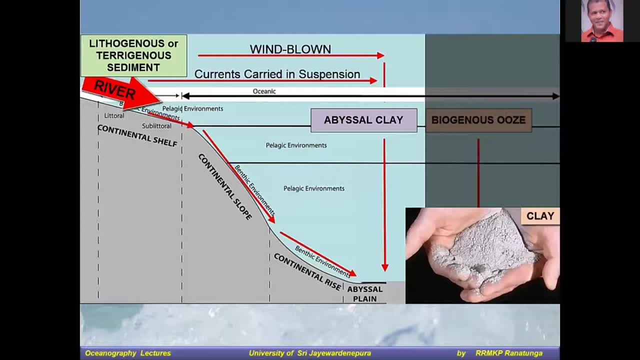 or by being carried by winds off desert and mountain areas. We call those clays abyssal clays, as they are found in abyssal plains. We'll return to them shortly, As lithogenous sediment dominates the coastal margins and accumulates at the fastest rates of all sediments there. 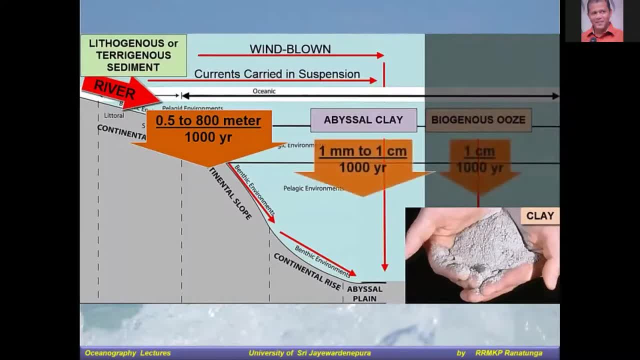 and also reaches out in its mud-sized form to the deeper parts of the oceans, predominantly as abyssal clay. lithogenous sediments make up the largest percentage by volume of marine sediments. However, because most of this volume stays close to the margins, 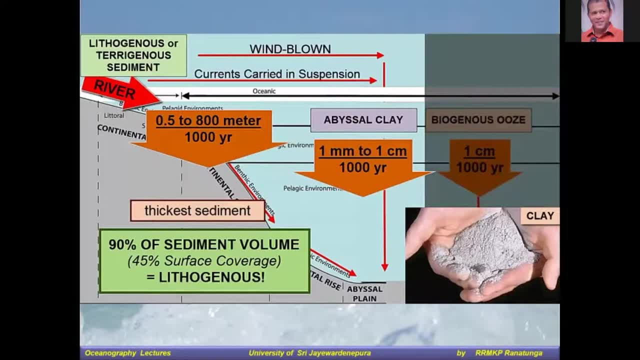 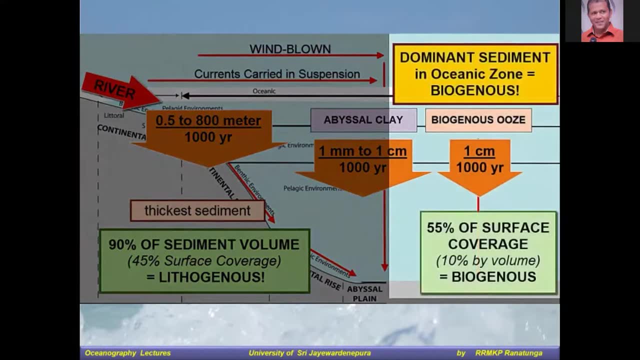 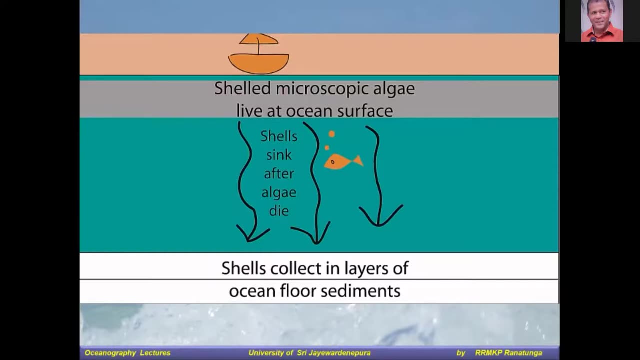 and piles up there thickly. they represent only 45% of the total seafloor surface coverage. The sediment that covers most of the seafloor surface is biogenous, which consists of shells of dead organisms and dominates the oceanic zones. 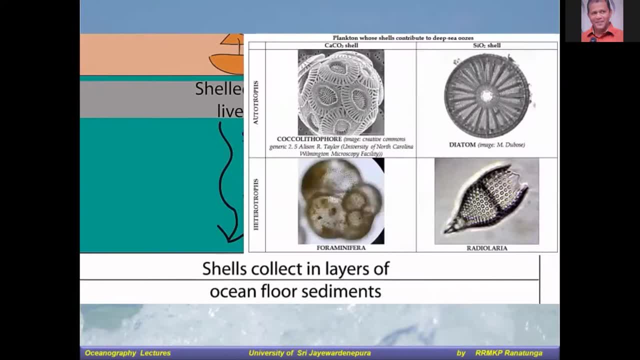 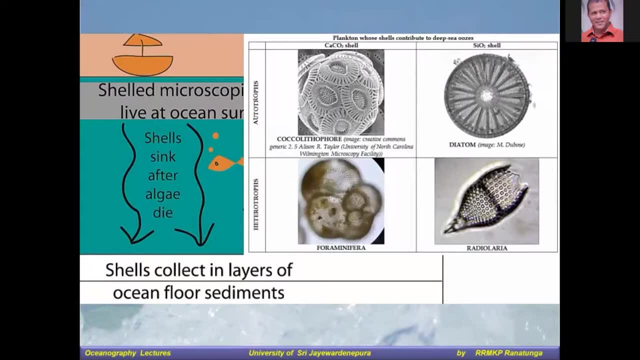 The most important contributors to biogenous sediment are the single-celled autotrophic and heterotrophic plankton that live in the surface waters. Billions of these organisms live and die, with lifetimes of days to weeks. Their shells collect on the bottom of the seafloor. 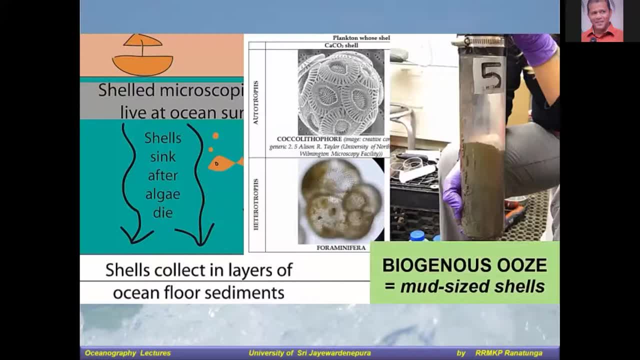 and contribute to siliceous and calcareous oozes, depending upon whether the shells are made of silica- siliceous oozes or calcium carbonate calcareous oozes. The term ooze tells us a lot about the consistency of these sediments. 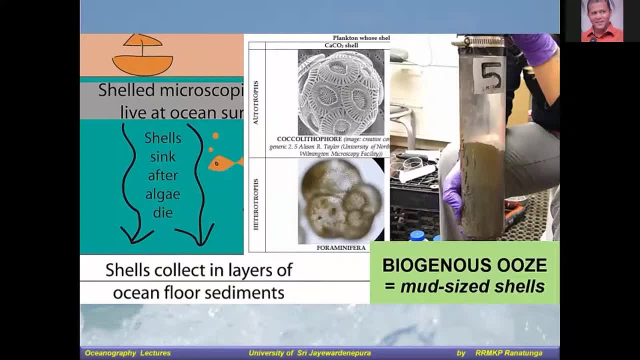 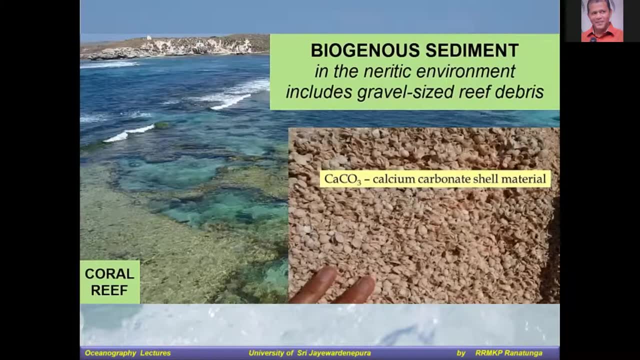 They are all mud-sized, a very fine flower-like material. Larger gravel-sized shells contribute to neuritic nearshore sediments where there are large reefs, either tropical coral reefs or colder water reefs made of mollusks like mussels and limpets. 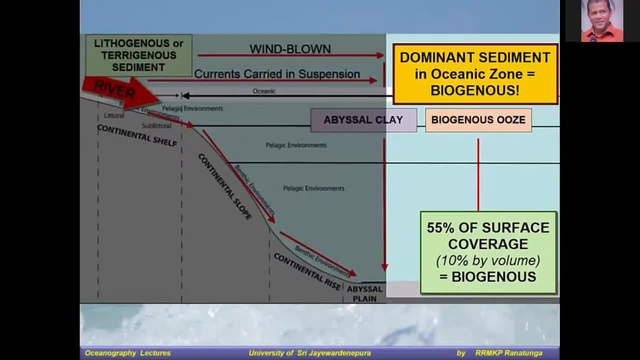 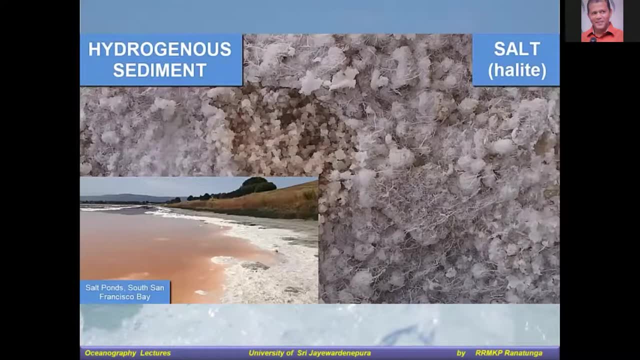 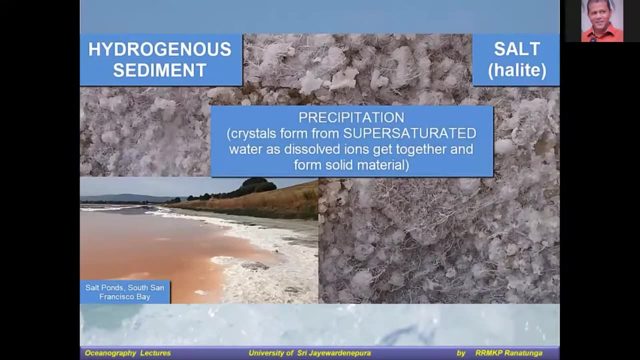 We'll return to the oceanic oozes shortly to describe them in more detail. Another type of sediment called hydrogenous represents minerals that are produced from ions that were originally dissolved in water. We call that process precipitation. Seawater has many dissolved ions in it. 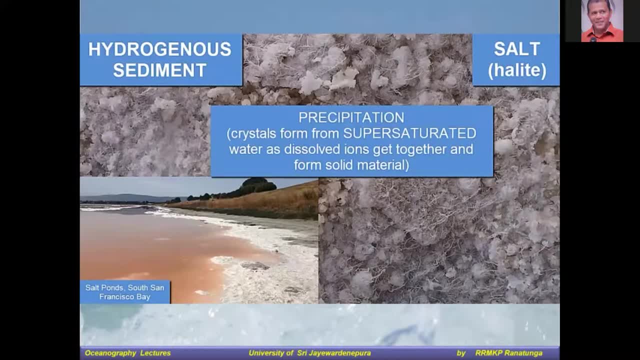 and in numerous locations those ions reach a concentration that is higher than can be dissolved by the water anymore, either because of evaporation of water or because of an influx of dissolved ions. We call that state supersaturated, and you can learn more about this in the seawater chemistry video tutorials. 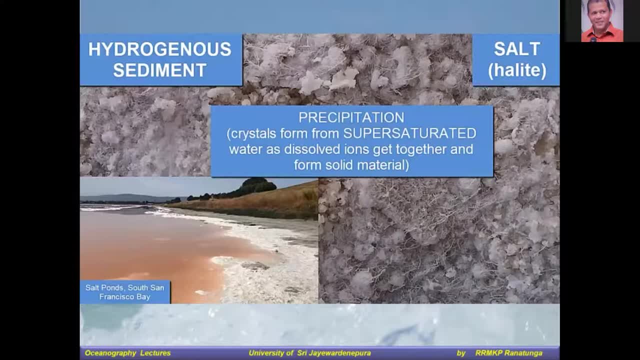 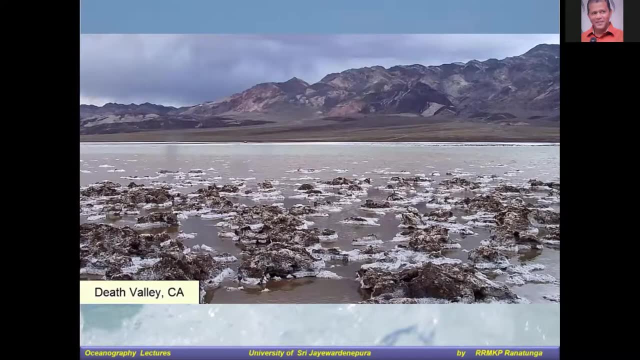 For now, we'll focus on where to find these precipitated hydrogenous sediments. At shallow inland seas, where rains are limited and evaporation rates are high, minerals can precipitate in high amounts. These minerals consist of halite, table salt. 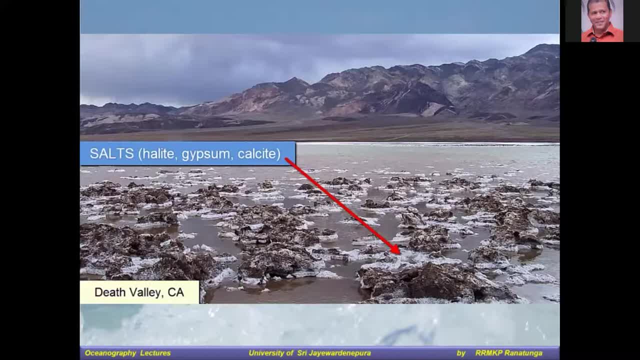 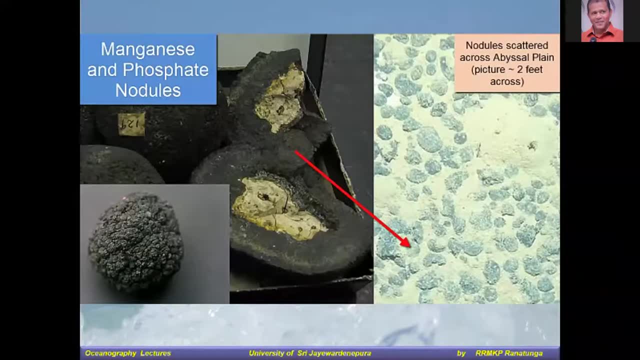 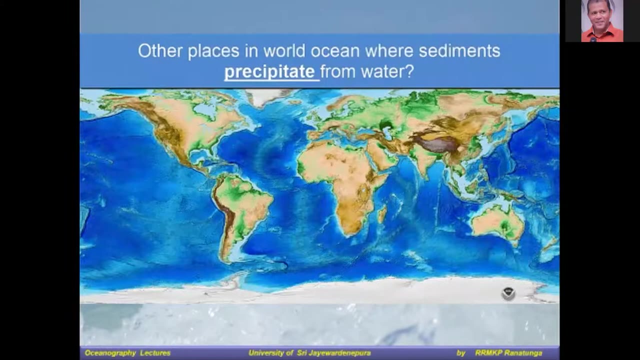 gypsum, drywall material and calcite. In some areas of the abyssal plains, dissolved phosphates and manganese become supersaturated and precipitate as nodules that grow bigger over time as new material precipitates atop the older material. Any other place in the ocean where sediment precipitates from solution. 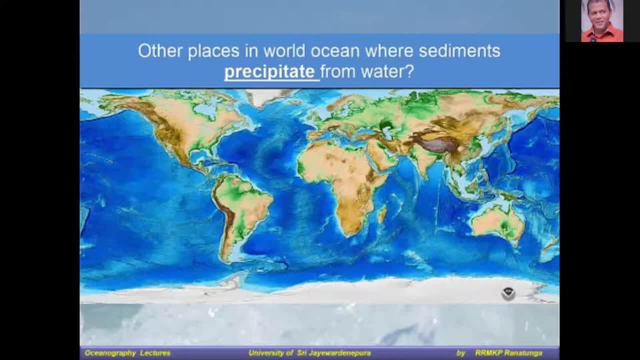 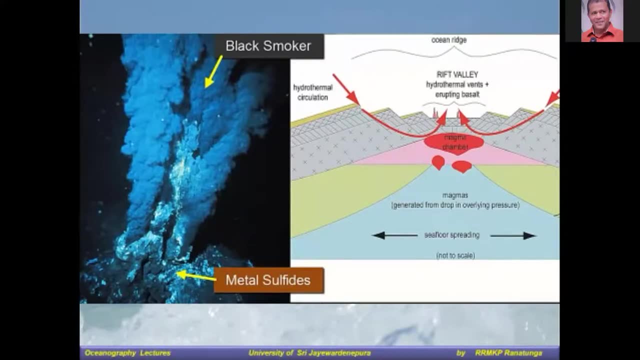 Something we discussed in the plate: tectonics and earth formation. video tutorials. Hydrothermal vents: Hot waters rich in dissolved ions leached from the ocean crust enter the colder seawater. As that hot water cools, it becomes supersaturated with dissolved ions. 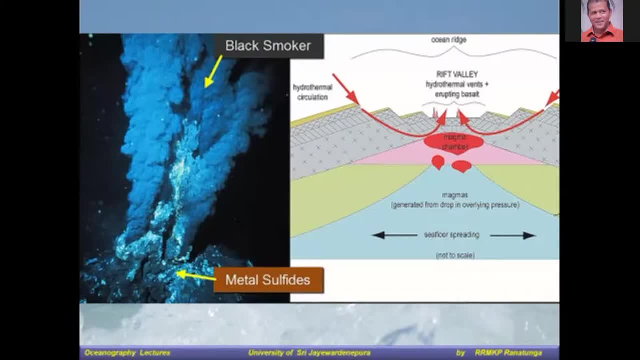 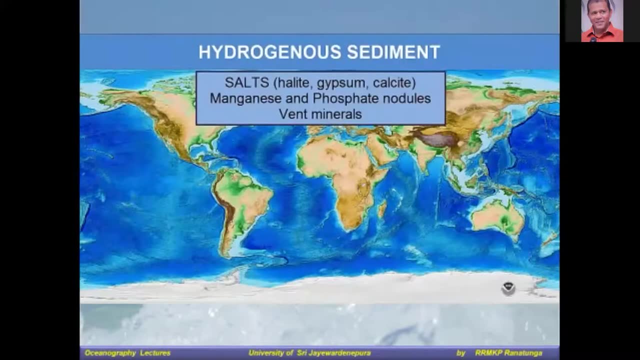 Cold water can dissolve less than warm water. That's why, when cooking, we heat up our water when we want to dissolve things like sugar or salt in it. Hydrogenous sediments are found in many places across the oceans, but they represent less than 1% of the surface area. 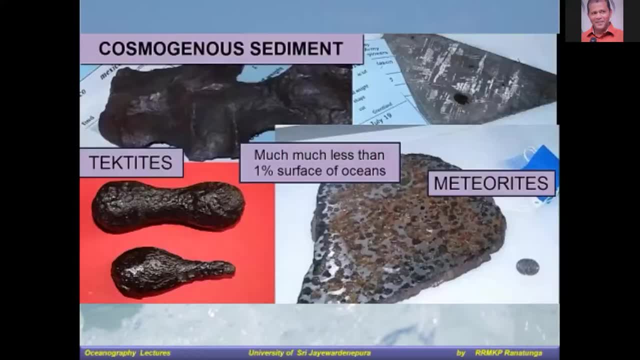 as they are largely scattered. The most uncommon sediment found in the ocean, but still found in abundances greater than on land, is cosmogonous sediment, meteorites that fall from space, and tektites which are bits of Earth's crust. 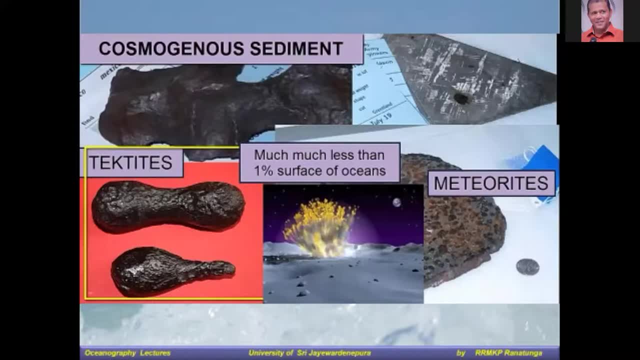 that have been ejected into space. after a meteorite impact excavates a crater, This ejected, excavated crustal material melts as it exits the atmosphere and solidifies as it falls back down, producing a spherical, teardrop-shaped glass nodule with eroded pits created by its journey back down through the atmosphere. 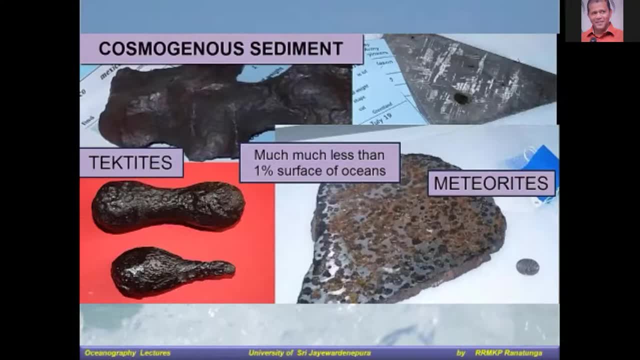 Why are these found in the oceans in more abundance than on land? Simply because of the slow sedimentation rate of the oceans, Where sediment collects at rates as low as 1 cm per 1,000 years, it's easier to find the tektites and meteorites that fall among them. 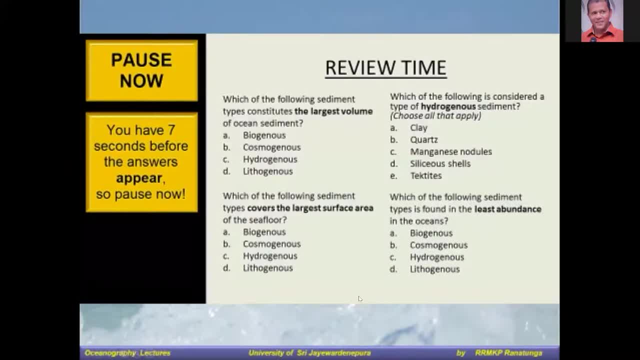 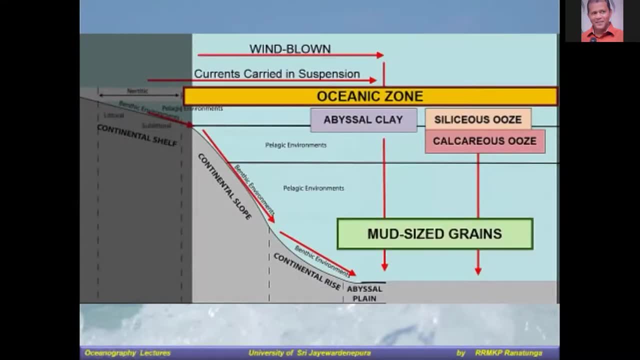 Pause, now clays, and siliceous and calcareous oozes that form. there Are all three found in the same location. In most cases one is the dominant, Why? Abyssal clays, remember, are lithogenous or pterygianous. 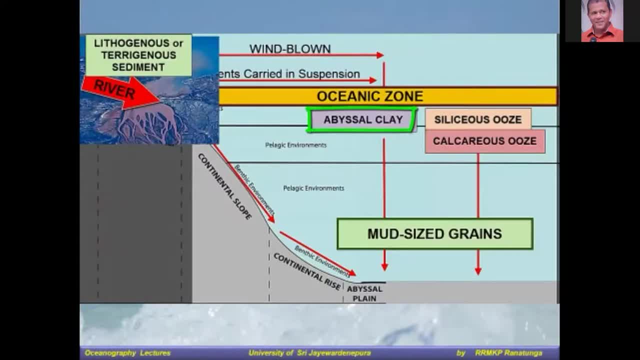 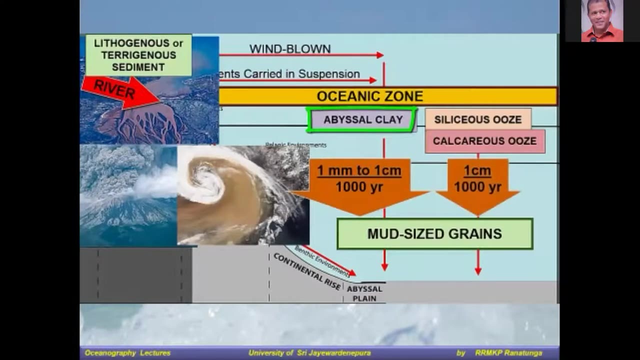 so they will dominate near high-volume rivers with large deltas Without rivers. nearby abyssal clays come from the settling of airborne dust and ash that's been blown from the land. If there are nearby deserts with high wind activity, the rates of abyssal clay settling can be comparable to that of calcareous or siliceous shells. 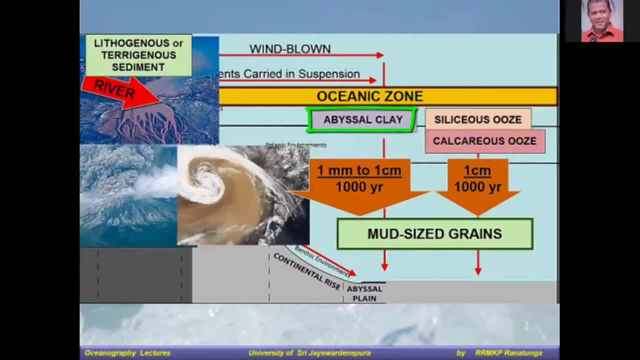 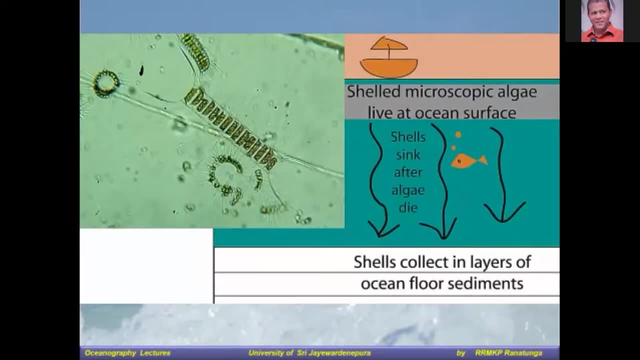 So the settling rate of abyssal clays in the deep oceans can be anywhere from 1 mm to 1 cm per 1,000 years. We call the organisms that live in the surface waters plankton Free-floating. can't swim faster than currents. 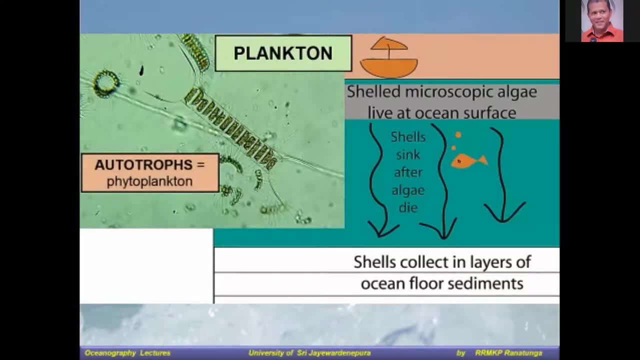 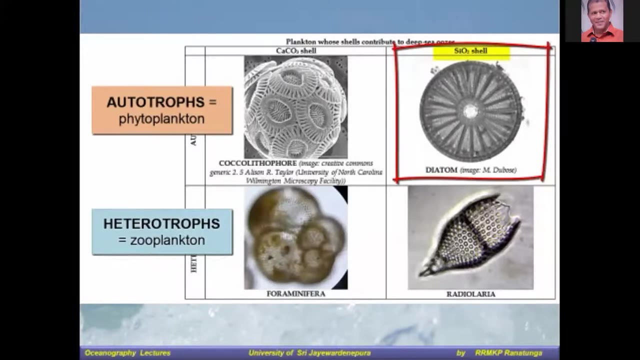 If they are autotrophic, make their own food. they are the bottom of the food chain and are referred to as phytoplankton. Heterotrophic plankton are referred to as zooplankton. Diatoms are phytoplankton with silica shells. 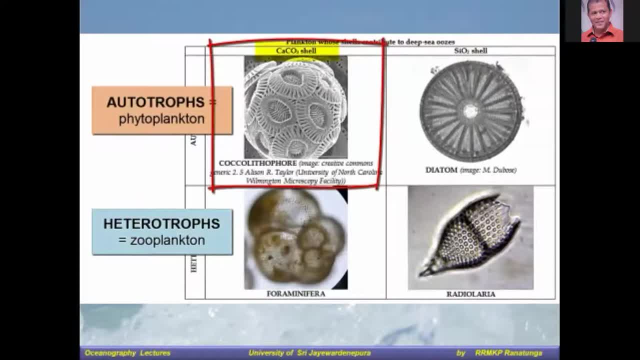 Cocolithophores are phytoplankton with calcium carbonate shells. Radialaria are the most common zooplankton with SiO2 or silica shells. Foraminifera are the most common with calcium carbonate shells. These four organisms play very important roles in the world's oceans. 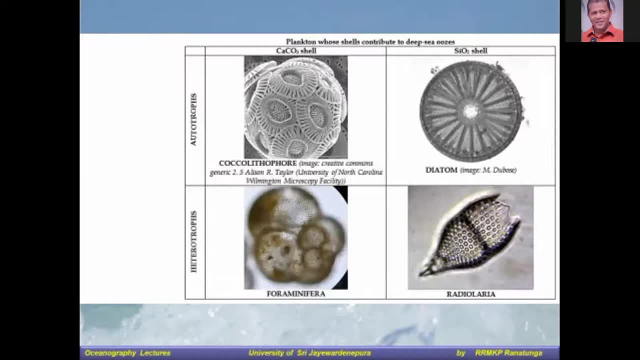 and it's valuable to memorize these names and shell types now as they will appear many times throughout future video tutorials. We'll review one more time. then you'll take a quiz. Autotrophs, diatoms and cocolithophores. 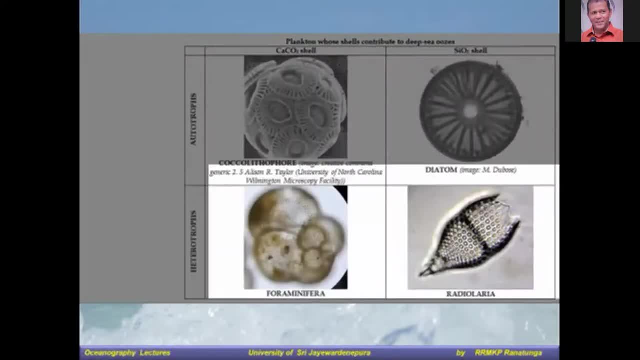 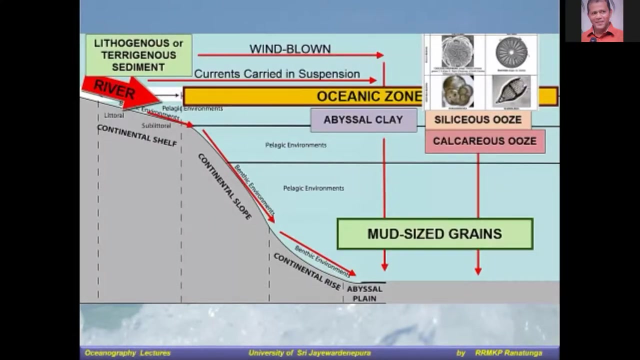 Heterotrophs, radialaria and foraminifera Silica shells, diatoms and radialaria Calcareous shells, cocolithophores and foraminifera. Pause. now Do these organisms thrive, and hence their shells dominate the oceanic muds on the sea floor. 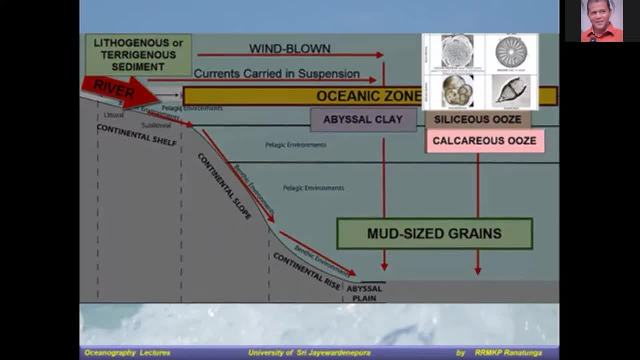 Calcareous shelled creatures are the most abundant organisms in the world's oceans, so theoretically, their shells should dominate all deep sea muds. That would be true except for two things. First, in areas where deep water rises to the surface, a process called upwelling- silica. shelled organisms thrive. These waters are cold and filled with nutrients. Nutrients are dissolved ions that autotrophs pull from the water to use for building cells and shell material. All autotrophs require that the water have nutrients. Heterotrophs get their cell-building and shell-building nutrients from their food. 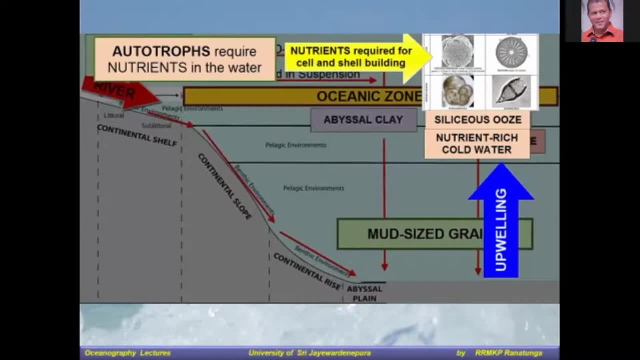 Since autotrophs make their own food, they need to get their nutrients from the surrounding water. Silica shelled autotrophs are adapted to cold, nutrient-rich water, while calcareous shelled autotrophs tend to prefer warmer waters. 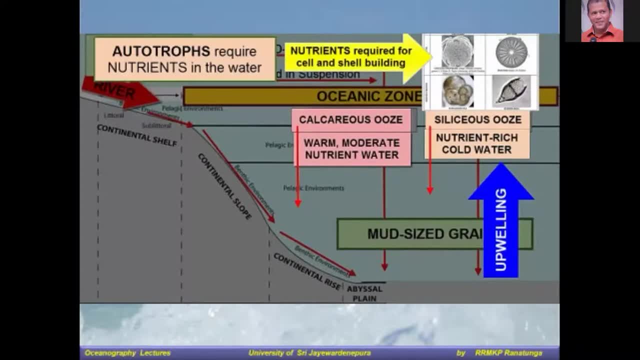 and don't require as high a nutrient content. So siliceous oozes dominate under areas of upwelling. Though some calcareous shells might also be found in these oozes, along with abyssal clays, the siliceous shells dominate. 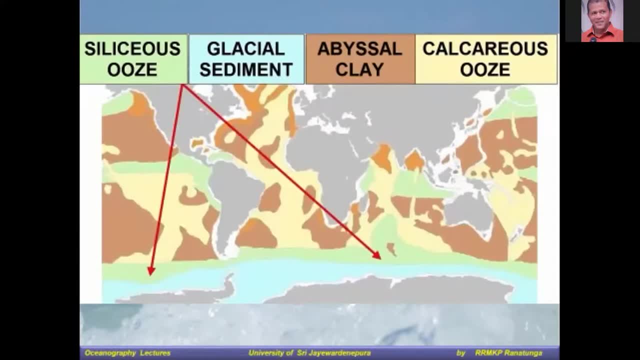 Where are these areas? Upwelling can occur anywhere at any time, but it is typically found year-round in the waters surrounding Antarctica and along the eastern edges of the ocean basins along the equator. We'll learn more about why that's true. 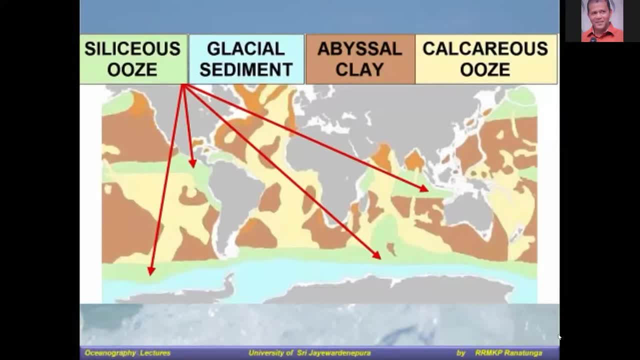 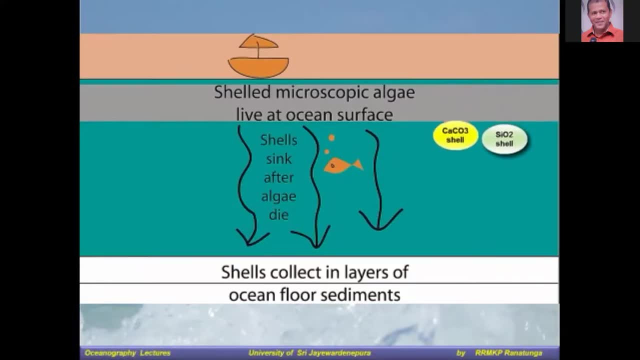 in the video tutorials that deal with ocean currents. So everywhere else there should be calcareous oozes- Not quite. There's one remaining issue to take into account: Calcareous shells will dissolve in acidic waters And as water gets deep. 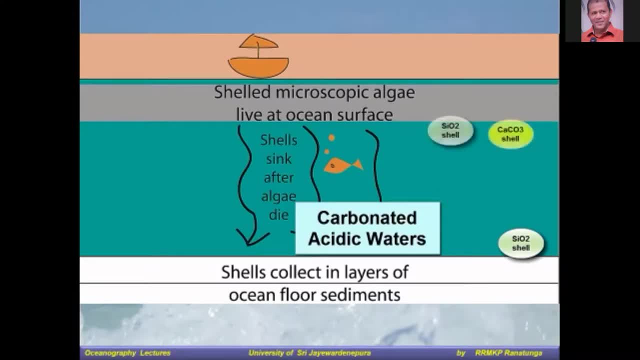 cold temperatures and high pressure mean more carbon dioxide is dissolved. More carbon dioxide means more acidic. For more information, refer to the video tutorial on carbonated oceans. For now, we focus on the result, Though calcareous creatures might exist in the surface waters. 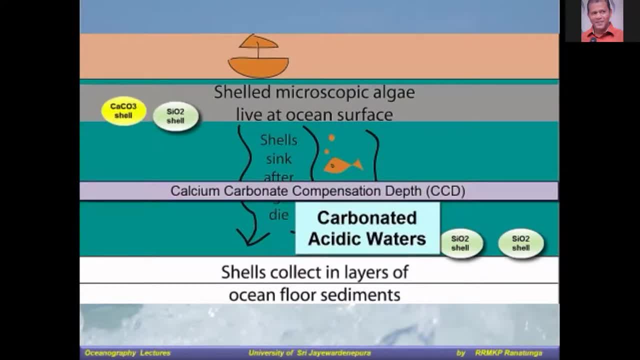 their shells will dissolve en route to the seafloor if the seafloor is deeper than the calcium carbonate compensation depth, otherwise known as the CCD. The CCD is the depth at which the acidity of the seawater is high enough to dissolve these shells. 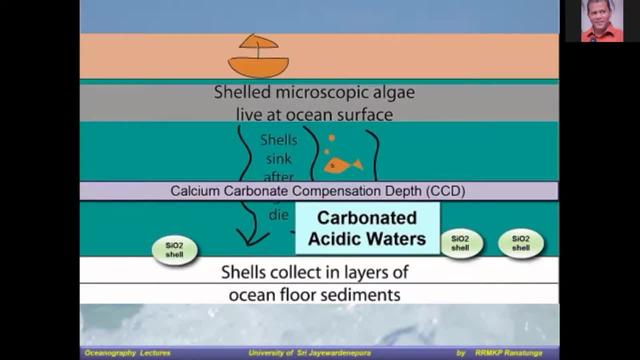 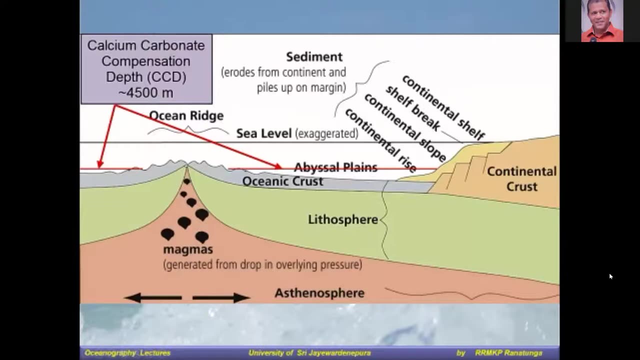 in their normal abundance, and thus no calcareous shells accumulate below this depth unless they collect faster than they can dissolve. For our purposes, that means they should be absent. This depth varies in the oceans, but is on average around 4,500 meters. 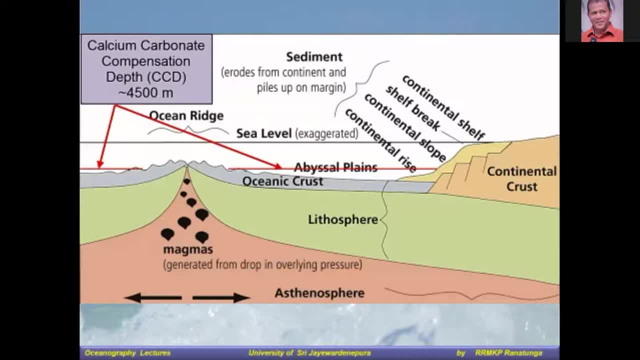 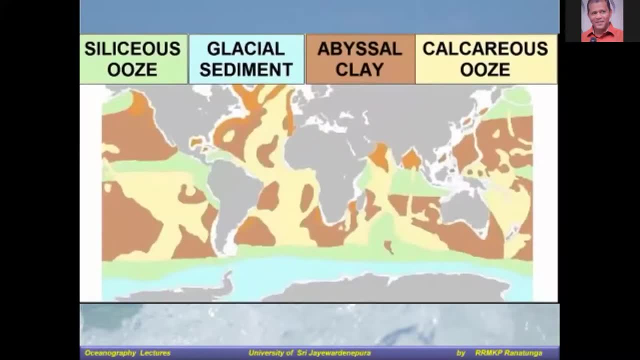 That means the deep abyssal plains will not have calcareous shells accumulating. Only siliceous oozes or abyssal clays can collect at these depths. So let's use this information now to describe the distribution of oceanic muds across the world's oceans. 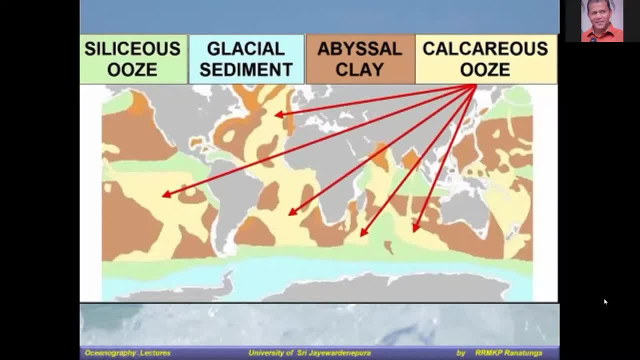 Notice the distribution. With what seafloor feature do these calcareous oozes correspond? Mid-ocean ridges, the shallowest parts of the oceanic zone. Siliceous oozes dominate at the eastern equatorial zones and in polar regions, as previously discussed. 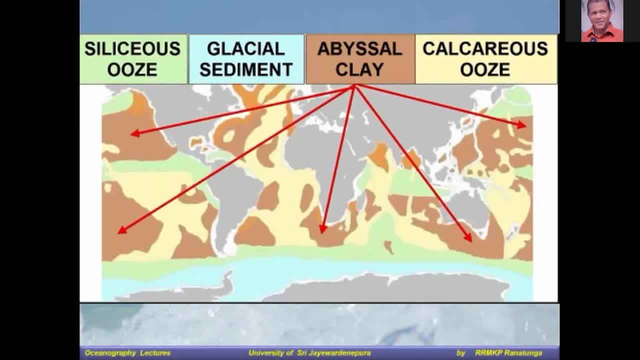 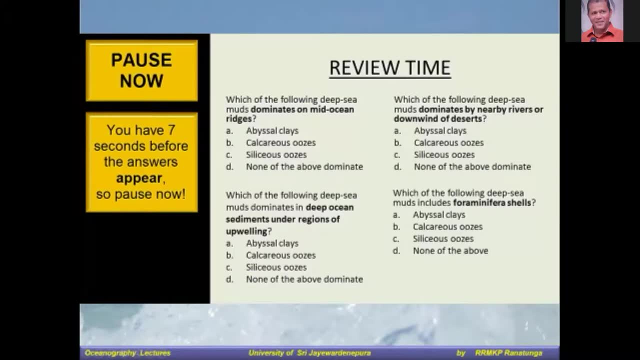 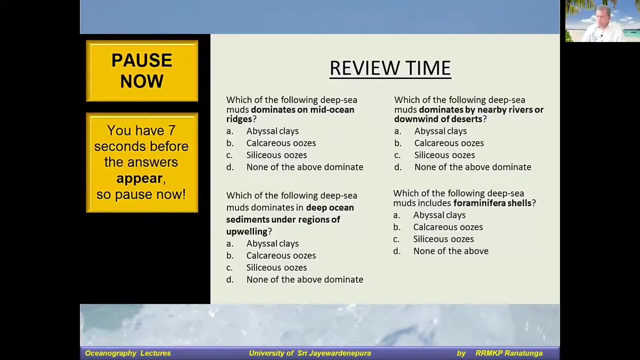 The rest of the oceans is dominated by abyssal clays. Pause now. All right, It might look a little bit too much for you perhaps. Actually, I just downloaded this video just before the lecture. before the lecture, even I seen this video, along with you. 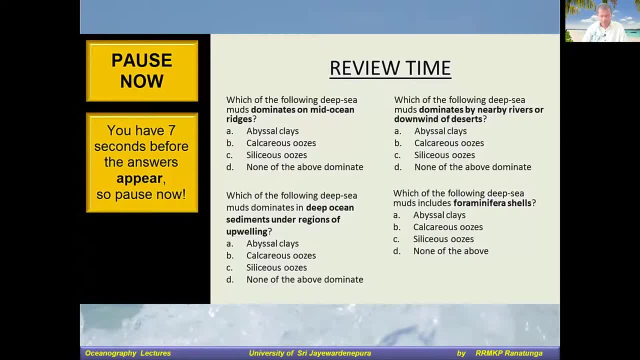 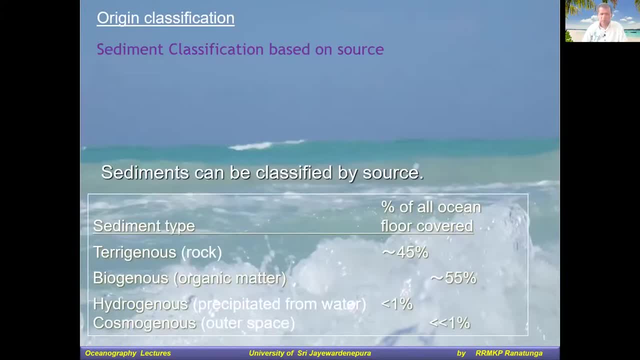 That described most of the thing actually related to the sediment basics thing. So that actually save a lot of time for us to go to the lecture. but I'll very briefly go through this: the types of sediments as well as the other metals. 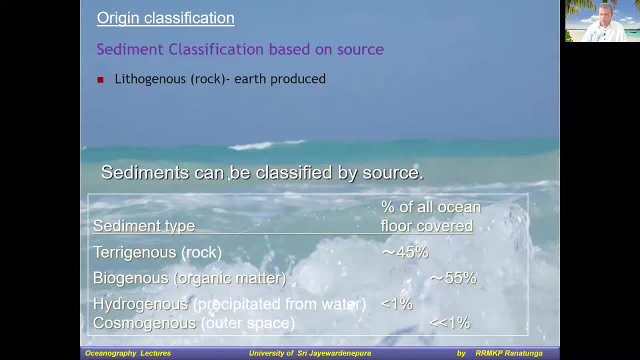 So, as we also discussed, basically there are four different types of sediments: a lithogenous or the- any sediments that form from the rocks, Therefore that there are terms that earth produce, because earth means the usually refers to the rocks. So the earth produce sediments and the biogenous organic matter. 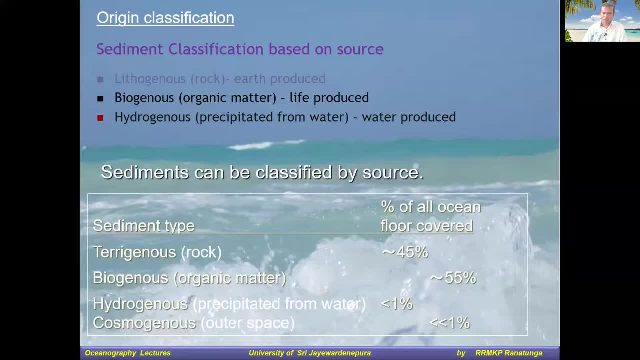 that's the life produce sediment, that the hydrogenous, that anything deposited from the seawater itself. So water produce sediment. and the last one, the cosmogenous or outer space universe, produce right, the simple terms. So that's how. these are the basic types of sediments. 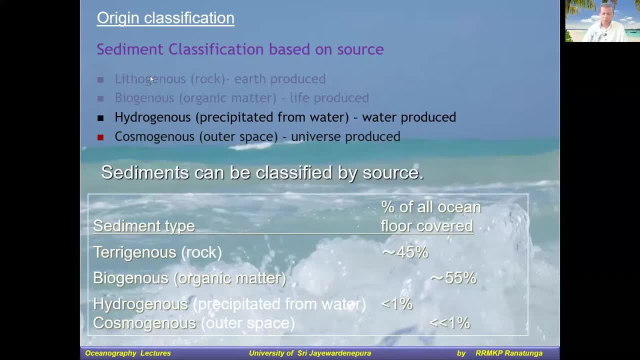 These are the types of sediment based on their origin, the how these sediments are formed. Here it's given the percentages, usually the how much ocean flow is covered. The terrigenous sediment is covered about 45%, That's cover. and biogenous sediment cover 55%. 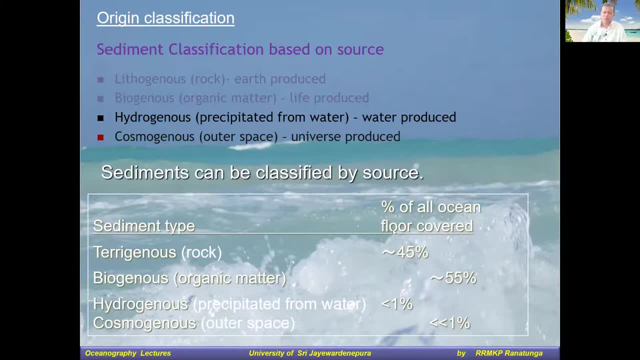 but the volume wise, there's a lot of terrigenous sediments because the volume is very high Compared to the others, right? So, as I mentioned before some the classifications, they talk about five different sediments, like a terrigenous sediments, biogenic. 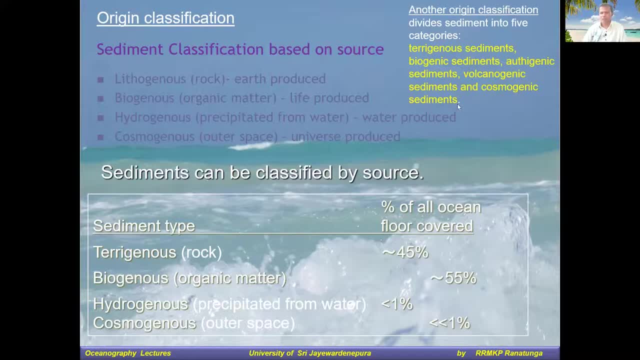 autogenic sediment, volcanogenic sediments and cosmogenic sediment, but it's not very autogenic, something like a sediment naturally built in the naturally formed sediment. So it's not formed in the ocean. And the volcanogenic are the anything derived from the volcanic activities. 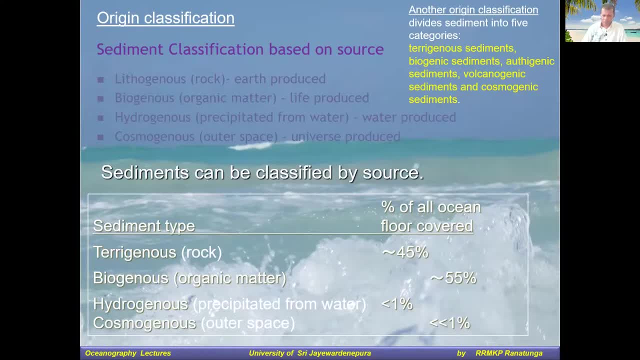 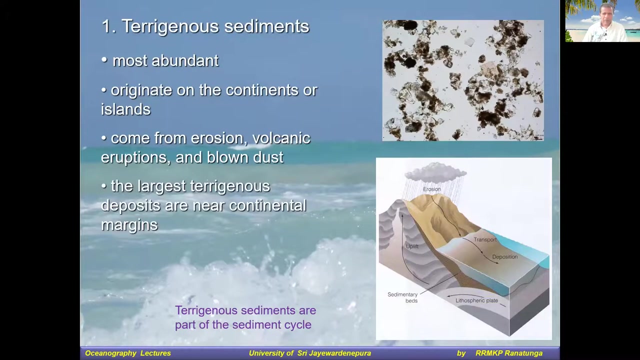 But again, volcanic activities also some sort of a earth produce sediment. So there's no much science here, So we'll stick into the other classification, right. So very basic. very briefly, we'll go through like a terrigenous sediments. 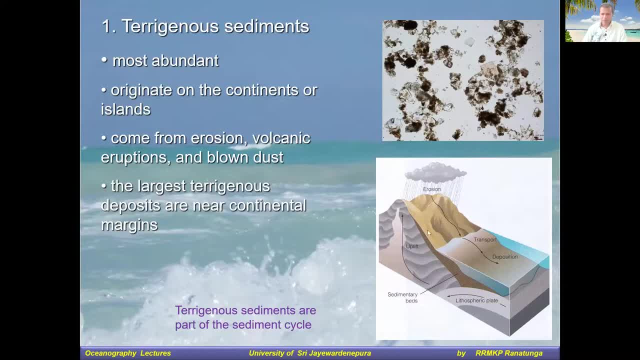 It's the most abundant sediments, And then they come from the, either from the erosion or the weathering of the rocks, and also the volcanic eruption, as you can see here, the volcanogenic sediment. there's no science again, because it's a part of the terrigenous sediment. 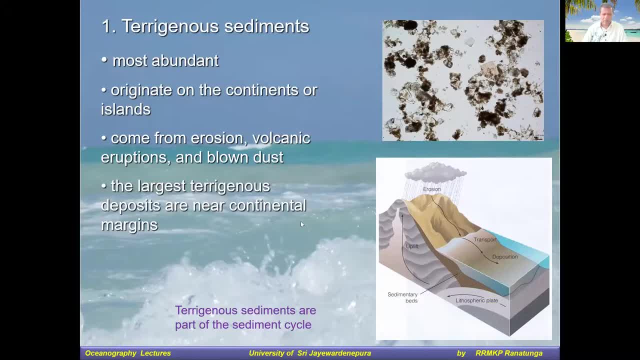 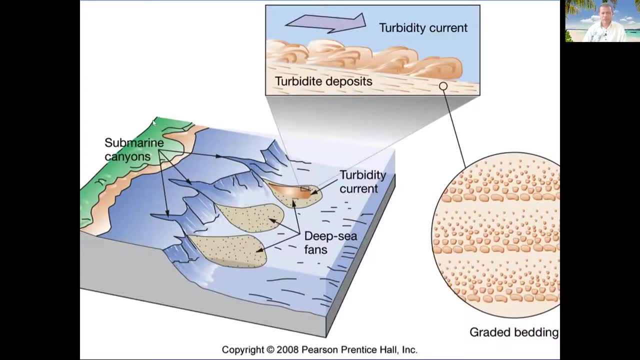 So what we? our classification is much better, right? So, since you already know, these sediments are taken to the sea from the mainly from the rivers, and then deposited in the continental shelf and even go beyond that to the turbidity currents or the turbidity deposits into the deep water. 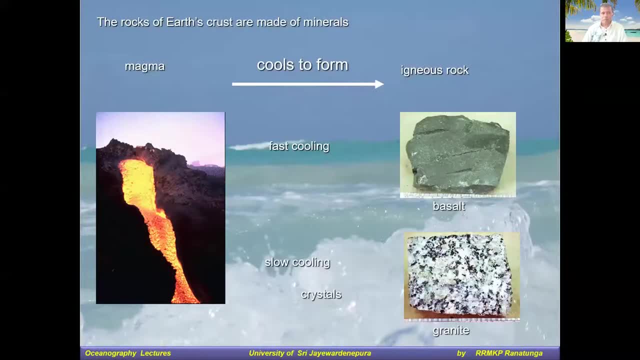 So we should already know, You may know that already this: what we call the rocks now, what we call now, what we call the sediment, the rocks, actually they can be like a granite or base, or actually they are originally the magma. 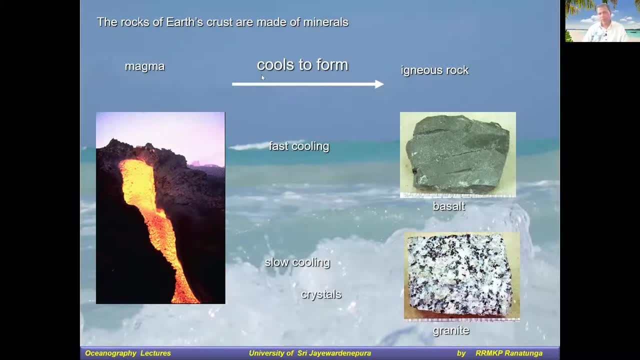 Magma cool. will see the level of call. Let's see. Maybe Ignis is a rock We're about to put. We're a vegan Cool, Not my base. What about what I'm not telling me? 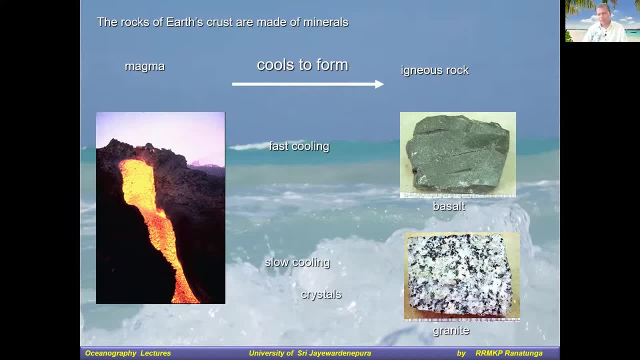 I mean cool, Call it. Is it cool? I mean granite Call, See, Yes. So again, we're all about the basalt, Yeah, but how about what I'm telling you We have. what was the question? 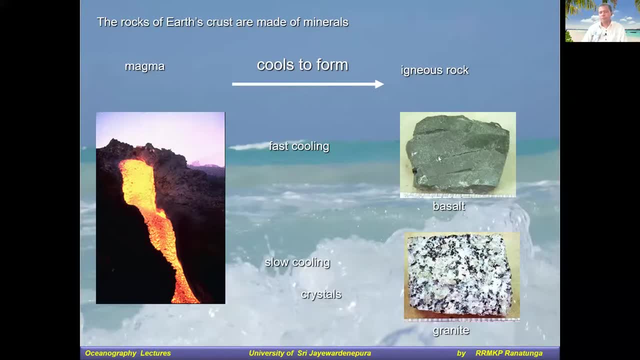 The question I have based on what we're talking about, Dancer basalt, I don't know, Granite to the continental cross. They're going up in the middle. Yeah, Then move. Did you want to? you know? would they want to run? 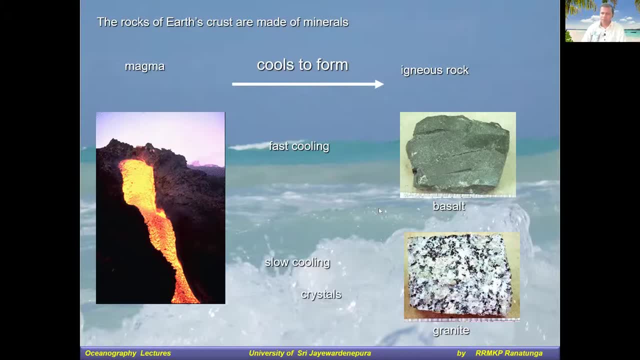 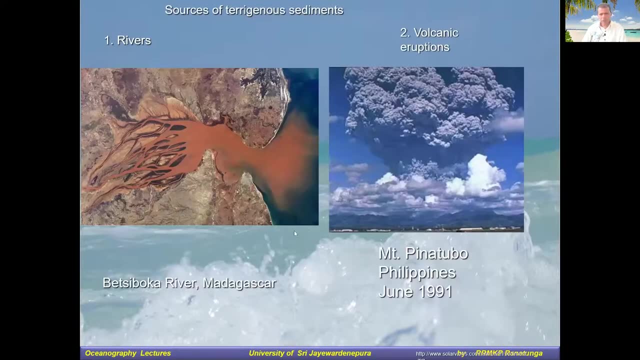 They, you know, they, you know, they, you know they're going to. Yeah, Anyway. so the ocean, get this terigenous sediment, or the earth produced sediment from rivers like here, and the volcanic eruption and the, as we discussed before that, the blown dust. 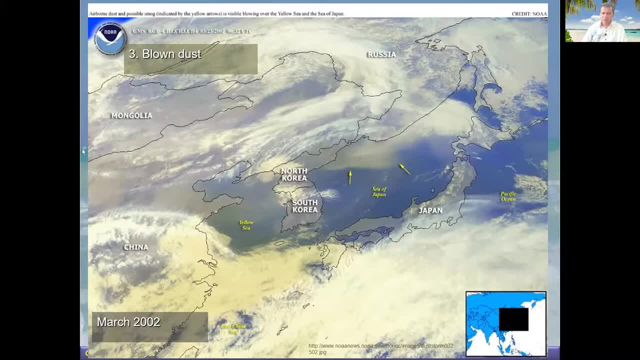 or the that dust carried from the wind, they can go across the ocean and deposited, And this is one example. you can see on the satellite images some blown dust through the Gobi desert, just above China and Mongolia. Gobi desert again, Haratini. 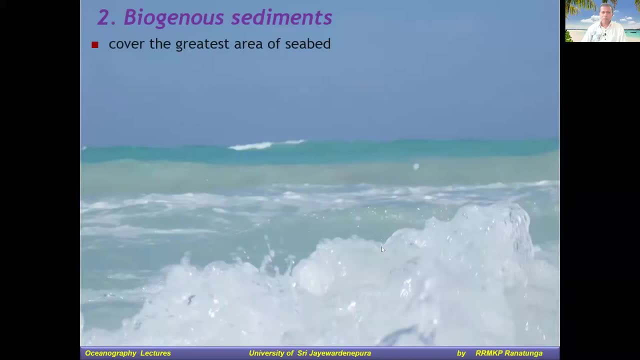 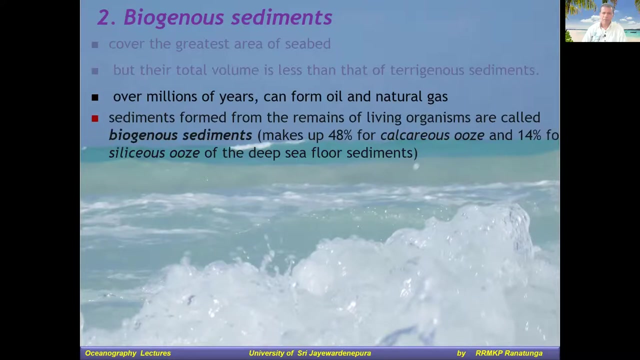 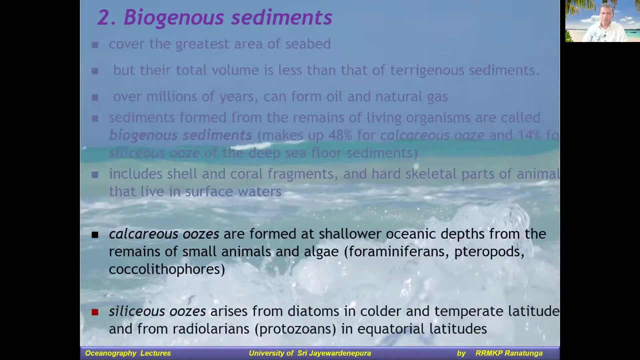 So they become terigenous sediment or the heterogeneous sediment right. So that second type is the biogenous sediment, So they are the the sediments that deposit from the activities of the marine organisms. So there are two types of the Biogenous sediments. they are calcareous oozes, that's, calcium based, and the siliceous. 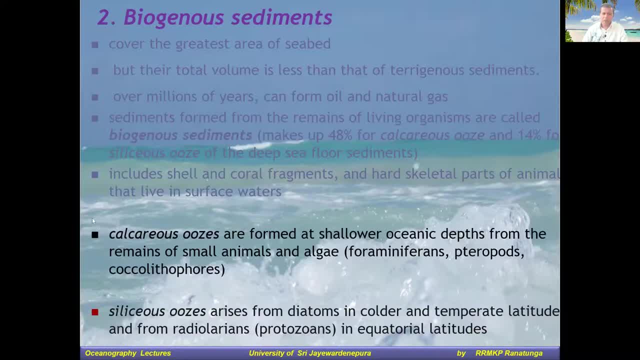 oozes or the silica based or the carbonate based. carbonate based oozes, called the calcareous oozes, and the silica based oozes we call the siliceous oozes, As you've seen from the video. Basically the calcareous oozes are formed from foraminifera. 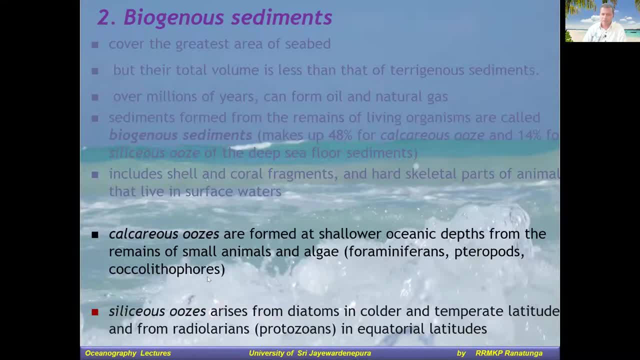 And some theropods, as well as coccolithophores, And then the siliceous oozes from the protozoans, and I think even the some algae also can form these siliceous oozes as well. Right, so that's how they are formed. 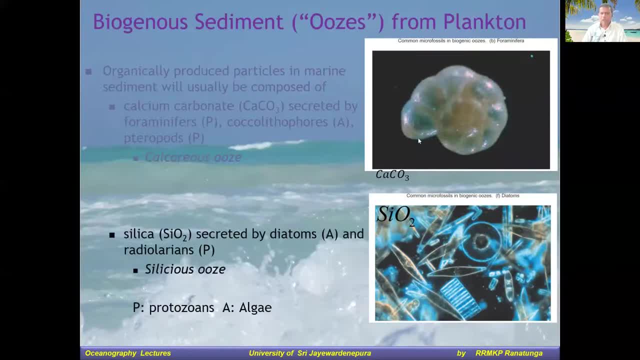 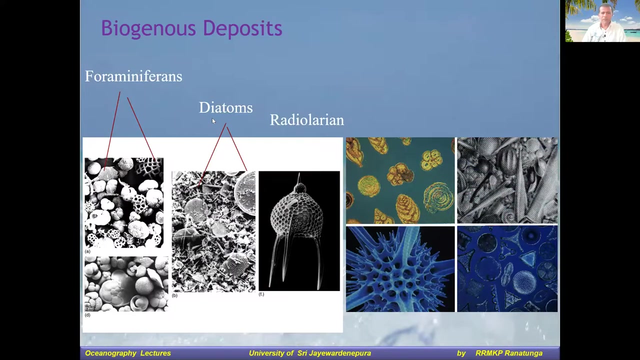 This is actually the, the calcareous oozes, or calcium carbonate, So Carbonate based oozes, and the siliceous oozes, or silica based oozes, Right So the, the foraminifera, diatoms, radiola and the other protozoans. they are the main source of these biogenous sediments. 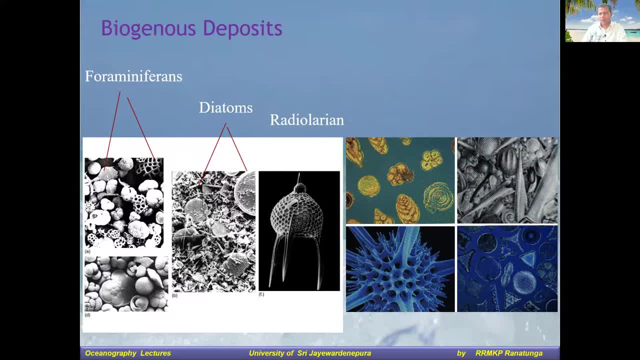 You can imagine how many of them they can deposit in Sometimes few meters to few kilometers deep layers of biogenous sediment. You can think of how big or how large plankton blooms can be. You can imagine the plankton bloom bloom skin. 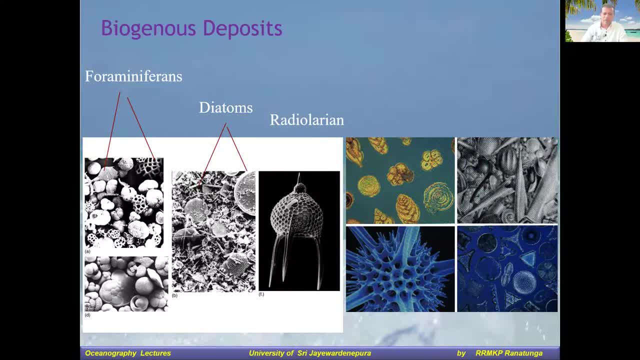 Somehow, a lot of them are a lot of some of the angle. It's all a bloom satellite And you can change that Bloom satellite. I mean Why? So that plumes are the ones that eventually become biogenous sediment, and once they are, 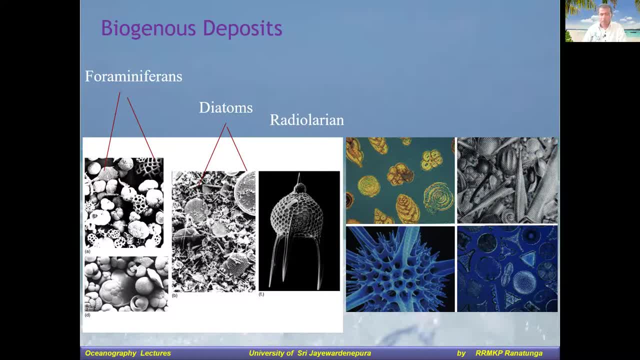 covered with the other sediments and over the millions of years they become. they can become actually not all biogenous sediments become oil and gas. if they have the right condition, right pressure and the right temperature, then they become natural gas or the oil. 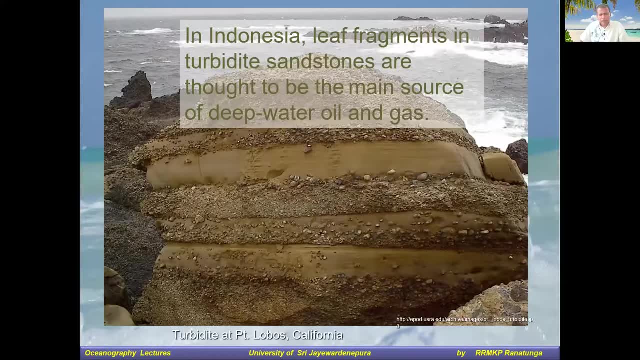 And this is an example. this is in Indonesia and this kind of a sediment called shale actually- okay, I'll try to translate this as shale. So shale, shale, shale. So this is a shale, this one is shale and this one has a different line in it, but this one. 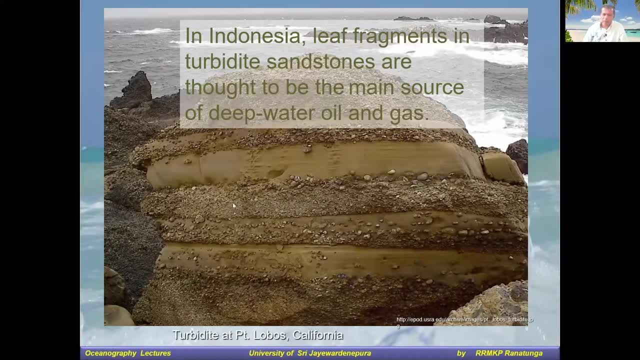 is a bit of a different kind of sediment. It is organic matter. These are biogenous sediments. these are other sediments. if I'm not mistaken, This is called turbidite. it is not just a black shell, it is also a mixed sediment. 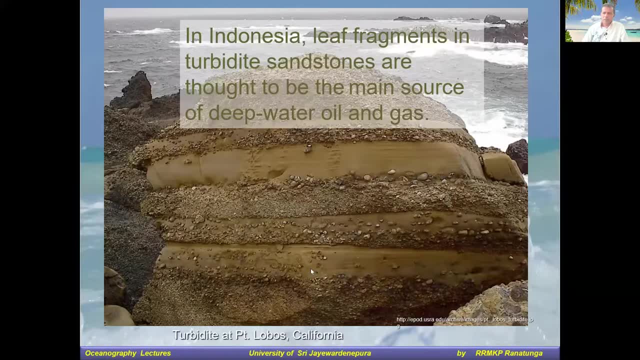 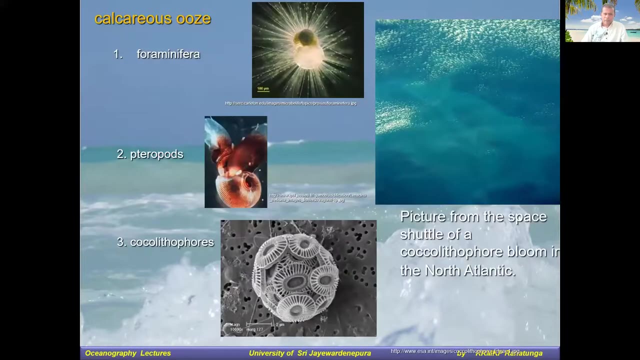 This is made of wood, but there is no pressure in the soil. This is made of oil and gas, but it is not made in this way. So these are some of the examples of the organisms causing this calcareous oozes. 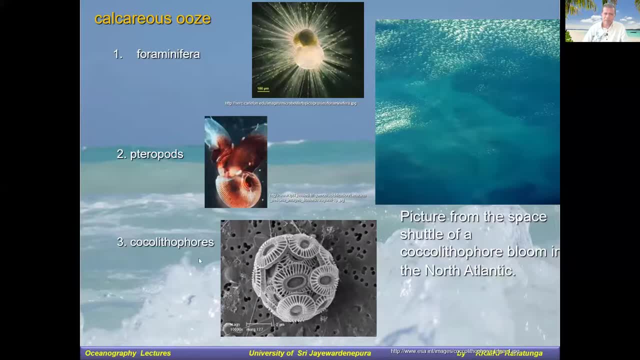 The foraminiferens, the pteropods and the coccolithophores. You can imagine this is a satellite image showing some coccolithophores. like these coccolithophores, They are very abundant in the ocean. 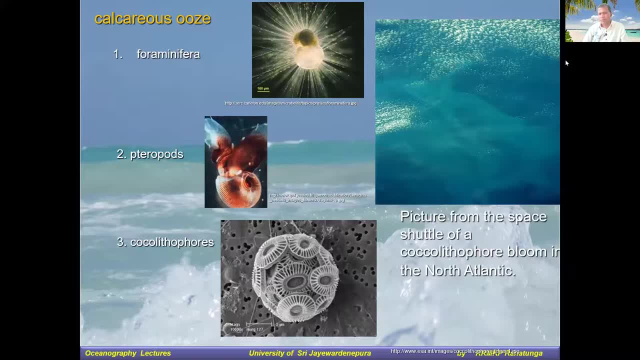 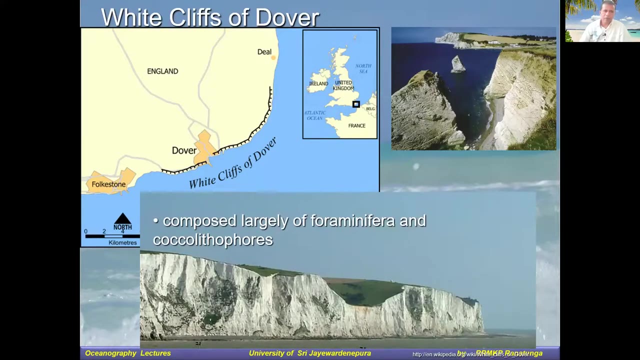 They can form large blooms. Even a satellite can detect their large blooms, So they are the ones that actually become a biogenous sediment eventually. This is one example. It is called the White Cliffs in Dover in the southern UK, somewhere here. 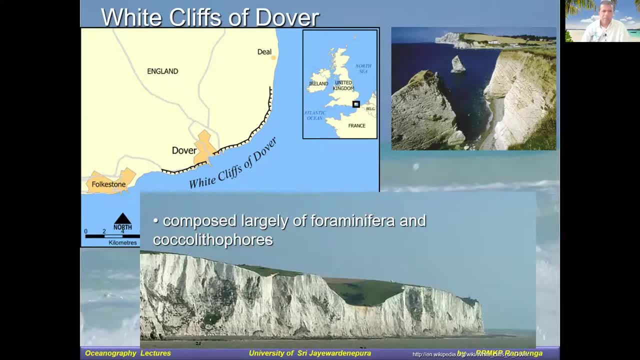 It is a very famous tourist destination. You can search in the internet. Search for the White Cliffs in Dover, Where this rock looks like white rocks. actually They are formed due to the biological activities deposited for millions of years. They have become sort of rocks- white rocks. 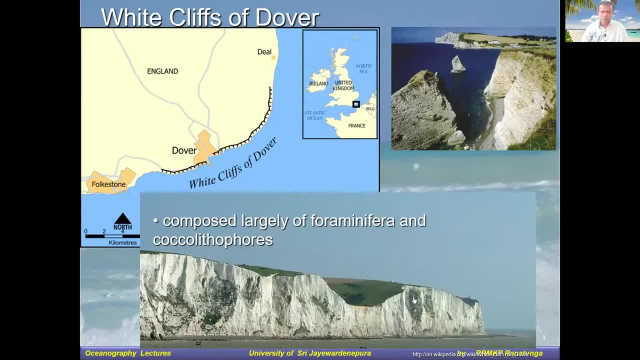 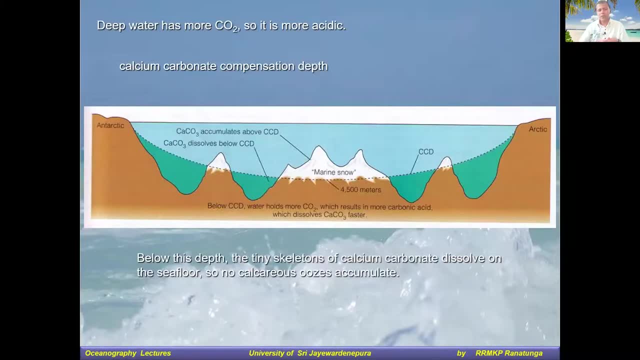 But they are actually the biogenous sediments. All right, And that video also talks something about this: carbonate compensation depth CCD. we call it, not the Coast Conservation Department CCD. This is carbonate compensation depth In the deep waters, as you may know. 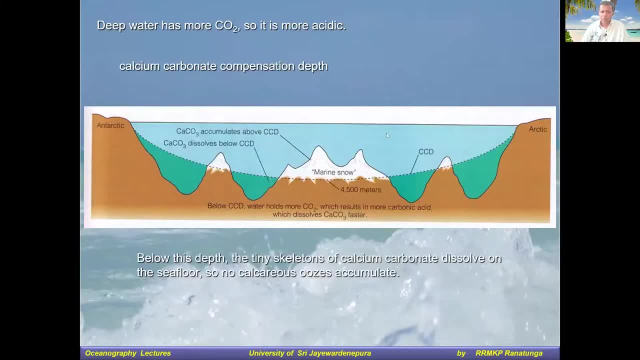 the the more carbon dioxide is dissolved. We know that the carbon dioxide gas they can dissolve easily under high pressure, Since in the ocean bottom, when there is a high pressure, there's a lot of carbon dioxide being dissolved And because of that, 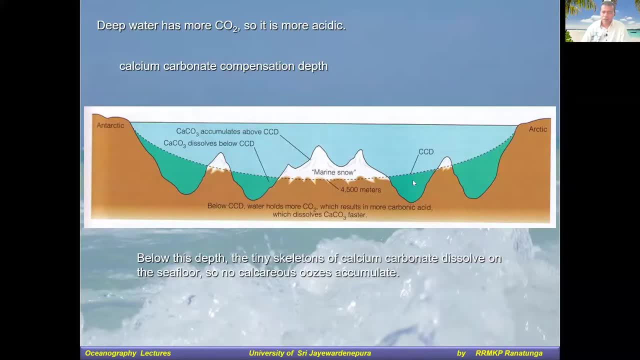 the acidity of the bottom was the water is very high And that's where the carbonates are dissolved. in that acidic waters Right And beyond this like a sort of a layer, the, because of the high pressure, more carbon dioxide is dissolved. 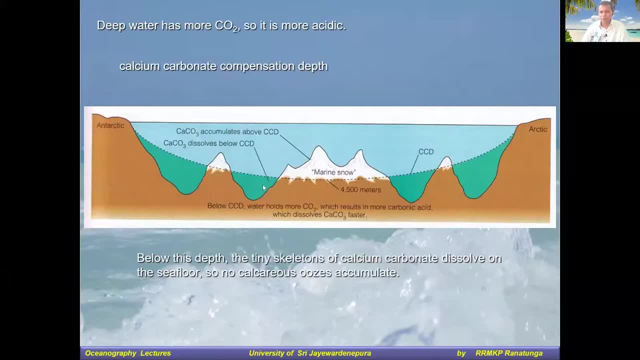 making the water more acidic, Right, And density is also high because this temperature is low. here The acidity is high And the density is high because of the low temperature. You know, when the temperature is low, the density increases. So then these waters. 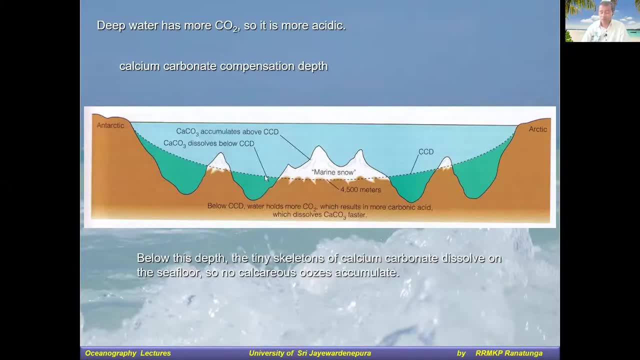 after this step, they will be the most of the carbon dioxide, So the carbonate will be dissolved And anything above this. the carbonate will be not dissolved very much And and that layer we call it calcium carbonate Or the carbonate compensation depth. 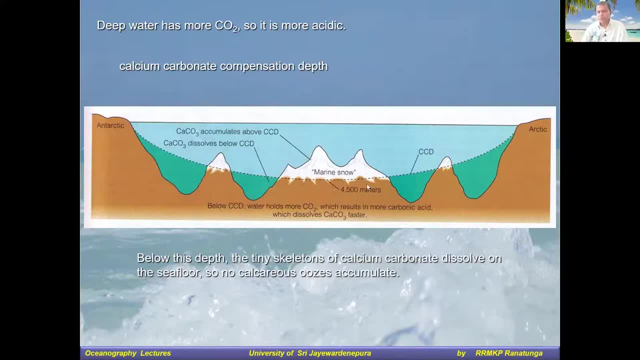 So that's we do also discuss it, like in the. in some areas you will have the deposited calcium carbonate, especially in the, when there is no enough depth or the not in the shallow areas, you will see more calcium carbonate or the carbonate deposit. 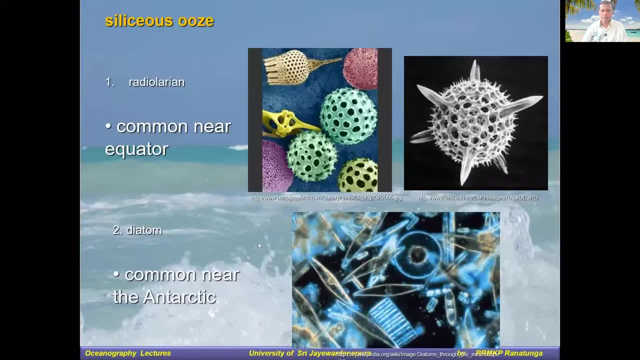 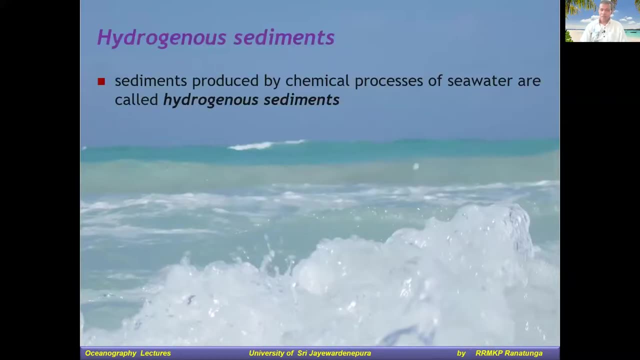 but not in the very deep area. So that's mainly because of the. they can dissolve, Right. So siliceous sources formed radiolariens and diatoms in this, a big case, right? So the third type of sediments are the hydrogenous sediments. 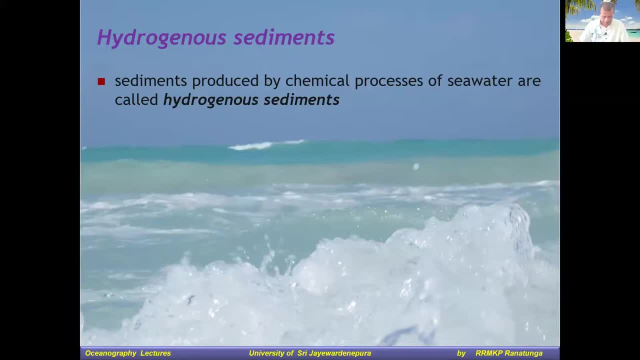 That's, sediments derived from the, the, the deposition of, from the seawater itself, So we call it precipitation from the sea. Some of the examples are the carbonates, as you have seen from that video, in some areas in the. 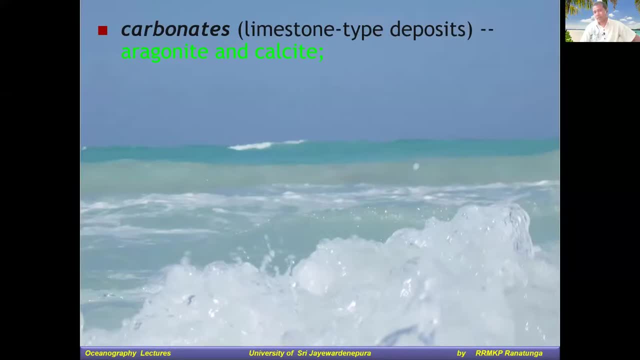 in the ocean, where this evaporation is high and the the fresh water inputs are low, When, in that case, they some of the minerals being depositing themselves, So they, some of them, are carbonates like this, arachnides and calcite. 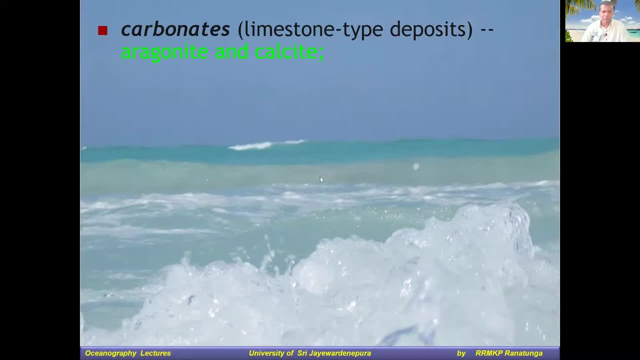 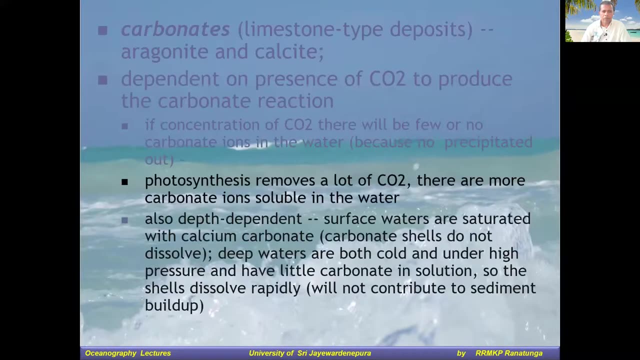 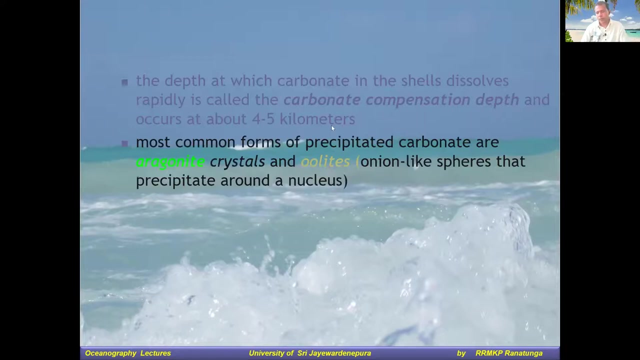 Just forget about these names, Just the geological names. And and then also other type of hydrogenous sediments are called you lights, One of the. You can even get deposited on some other time- a lot as hydrogen and sediment. 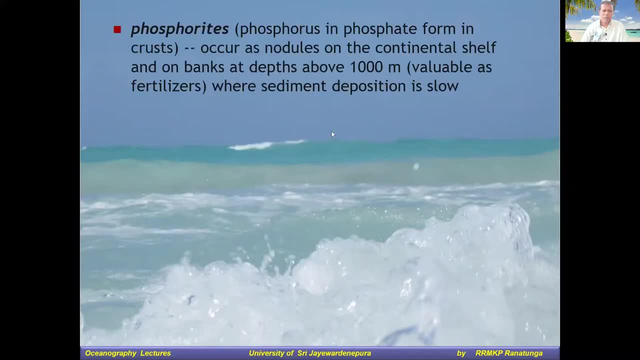 right. So the first perides. for the other example, they're all hydrogenous sediments In some areas in the ocean, a large deposit of this kind of a phosphorus or phosphorus base or phosphorite deposits. you see, then, if you have this kind of a large deposit in somewhere, it could be a really good source. 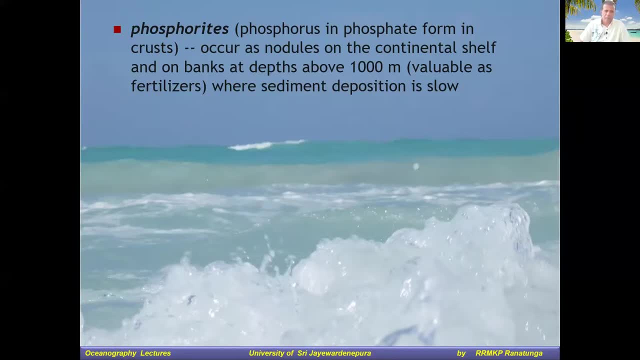 where you can manufacture fertilizers- we don't know- in in the ocean around our country if we have some like deposits of this phosphorites, and then that would be a huge source. so unfortunately, we could have produced some fertilizers of our own, but we don't have much nitrate sources, so we might need to import some. but 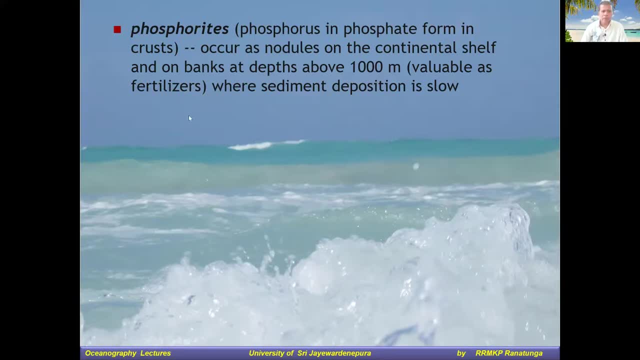 at least we have the phosphate, phosphorus sources, right, and the very important type of hydrogen and sediments we call the manganese nodules. manganese nodules- this is actually- uh, i show you have seen that- some of the images of the ocean bottom with- i told that- with some sort of a. 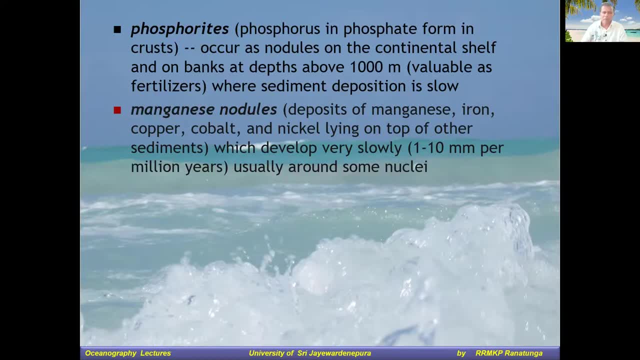 some pattern in the sea bottom that is because of the deposition of this manganese nodules. actually, even scientists has no much idea why and how these manganese nodules are formed. but like the mixture of some irons, like the, like some the metals, like iron, copper, cobalt, nickel, now they are, they become like together, making small balls. 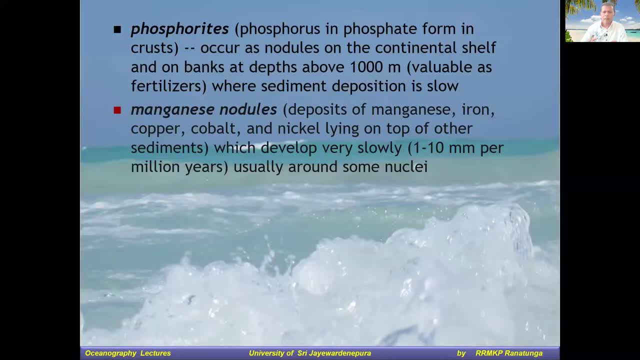 just like a potatoes. they can be larger or smaller than potato and they are deposited in a large amount in the ocean bottoms. they are being like. they can be one to ten millimeter by- i mean deposited annually- and they become like a potato size or even larger. 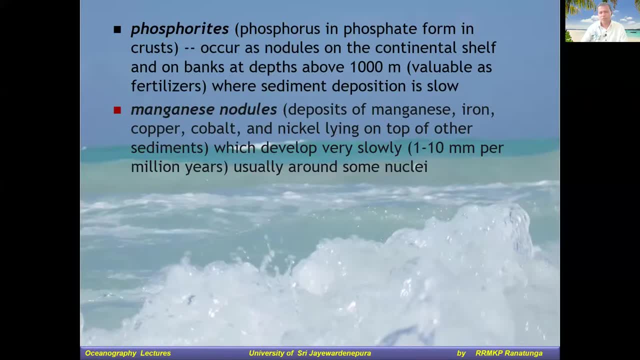 and they put deposited in the huge amount of these manganese nodules. some scientists say that these nodules start depositing around the, the teeth of the sharks. you might have seen other sharks slugging in the deep. you know this is the deposit of the sharks, but i don't know if sharks are there or not. 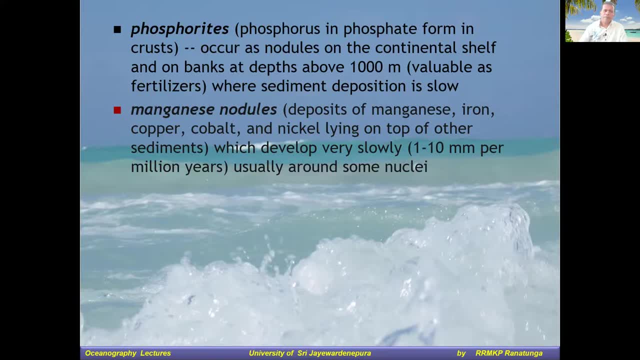 but anyway, um, no matter how they deposit, but you see if in our ocean, if you have this kind of manganese nodules in large quantities so you can extract them and then they can be a really good sources of manganese and nickel cobalt. i mean, they are very important um. 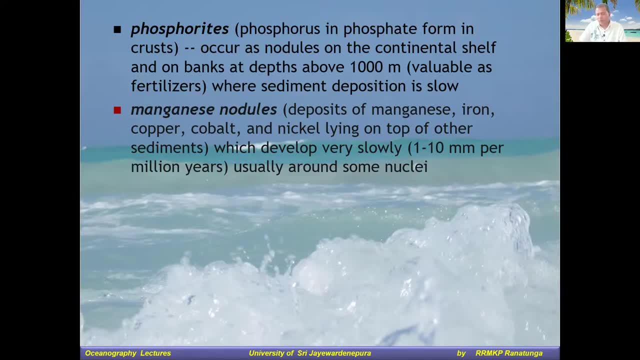 metals or the minerals that you can even export, but unfortunately these are in a very deep waters, several kilometers perhaps, so taking them to the surface going to cost a lot of money. you need a deep water explorations. it's going to cost for the moment, you know the the from the present market price which you are extracting these. 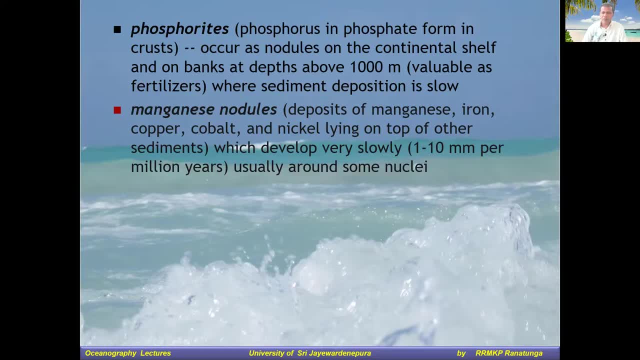 minerals from the ocean. yeah, the price will be several hundred times the cost then you extracting them from the the land. so not uh economical at the moment but uh in the future so they can be a very good source of uh that we can extract the earth minerals. 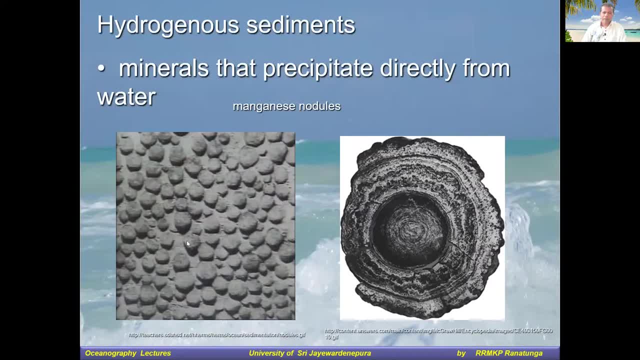 right, uh, here you see this, uh, the depreciation of manganese nodules, and this is a cross section of this: manganese nodules, how they are deposited layer by layer, um, um, and uh, yes, actually some of the countries already they are extracting this, uh, manganese nodules, but, uh, we don't know whether we. 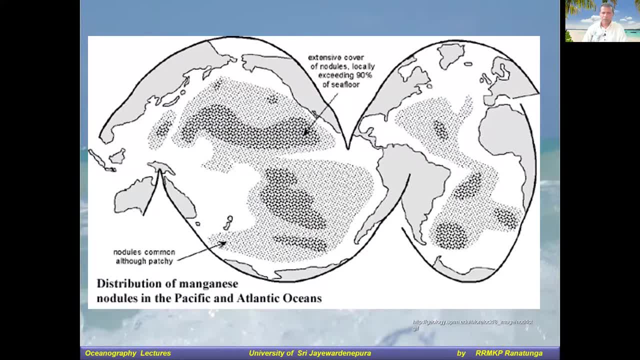 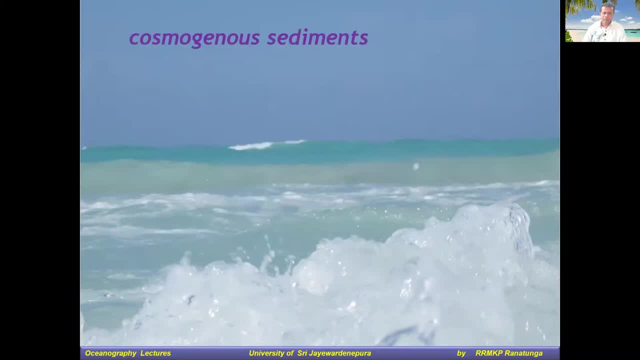 can extract this manganese nodules in around the the ocean, right uh, all right the. the last type of marine sediments are the cosmogenous sediments, or the. the universe produce uh sediments and they mainly produce from the uh meteors that uh that are. 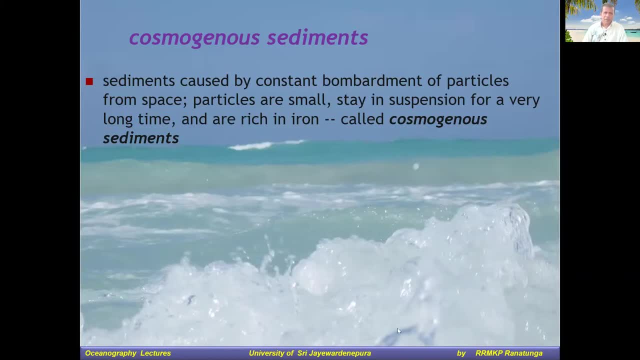 bombarded or the that reach in the earth, because every moment, you know, these meteors are coming to the earth but they, because of the resistance and the in the in the earth's atmosphere, they are just burnt and then make it a smaller, smaller pieces or they become actually dust and they are continuously being deposited. 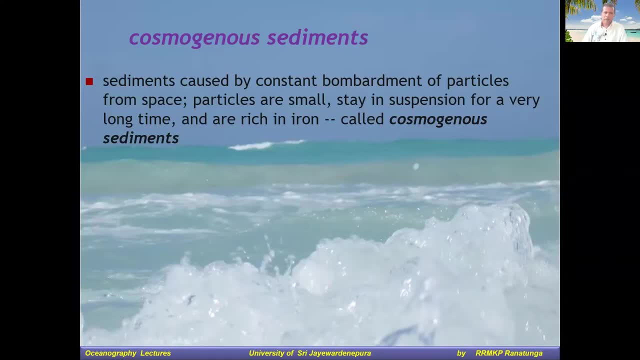 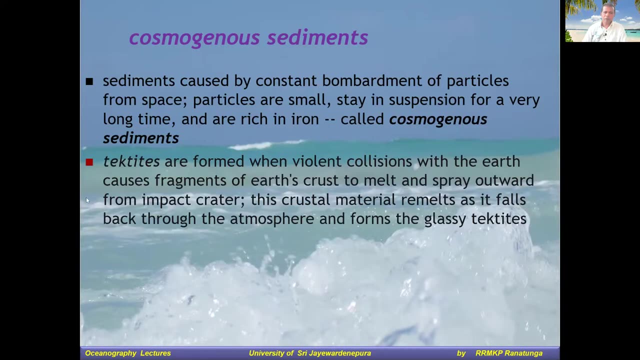 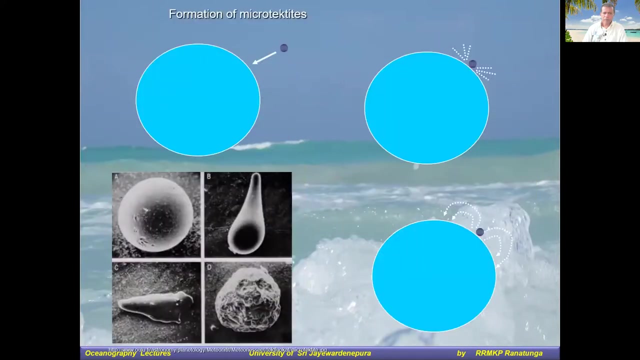 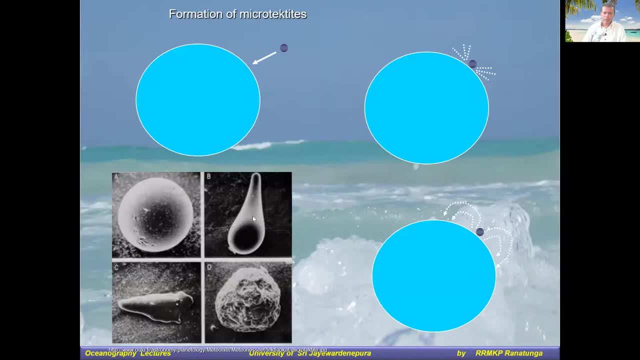 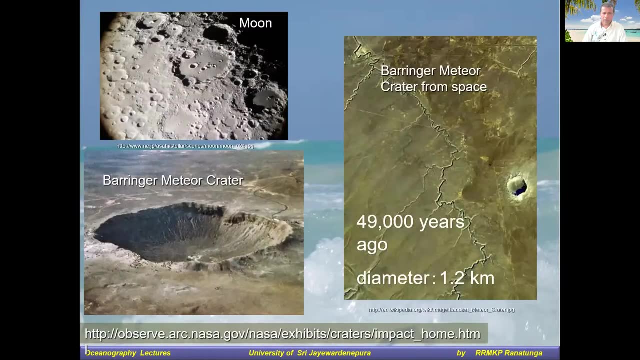 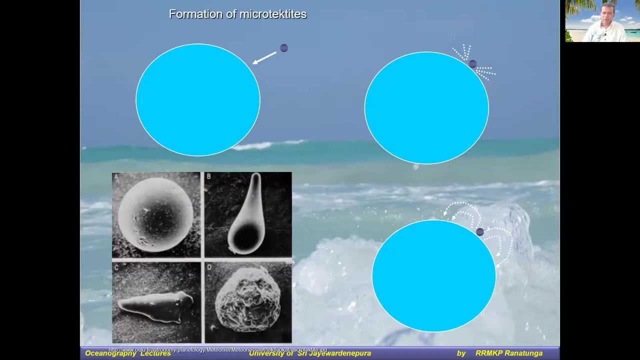 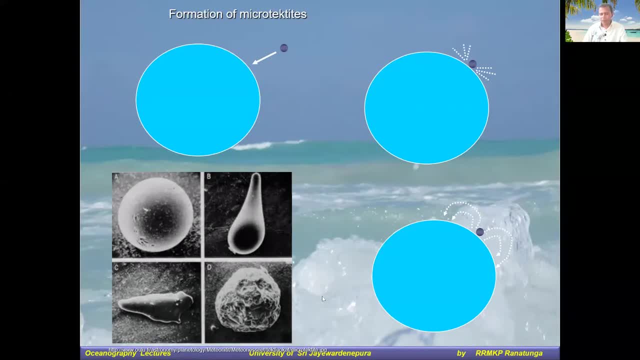 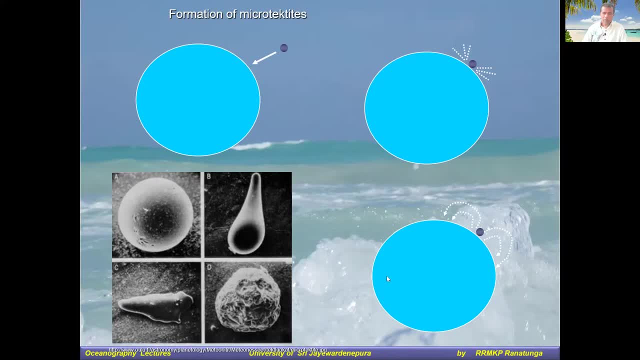 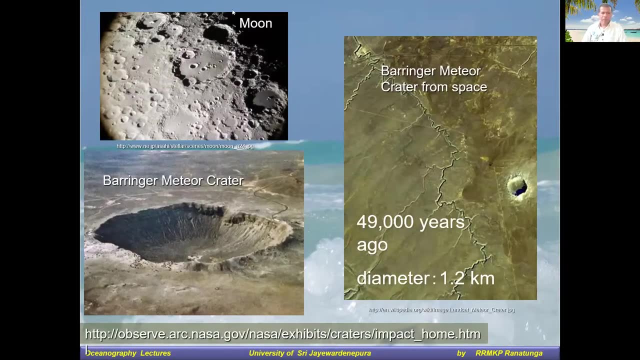 tektites, the exception of tektites kepa, For example. this is the Bering Meteor Crater. It is 1.2 km long. You can see from the satellite image that this is a meteor crater. You can see what happened to it. 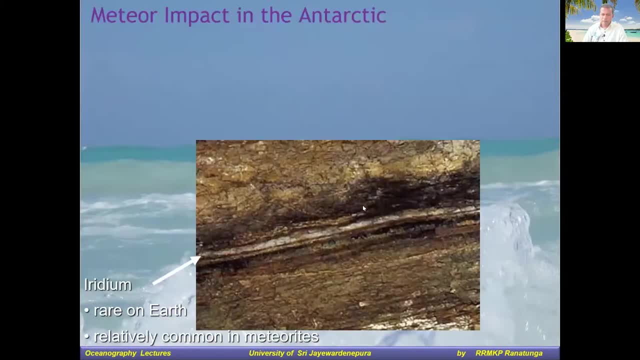 This is the same meteor, but the meteor is not visible to the naked eye. Here is the origin of the metal, Iridium. It is very close to Earth. This is because Iridium did not come from the earth. Iridium existed in other planets. 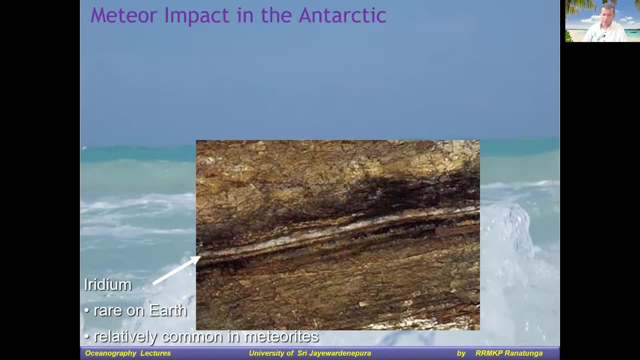 This is the Iridium that appeared in Earth. This is the Iridium that appeared in Earth. This is the Iridium that appeared in Earth. I don't know where it came from. I don't know if there are any more bloodstains. 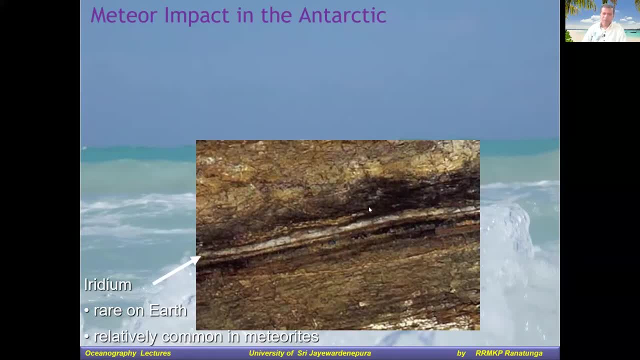 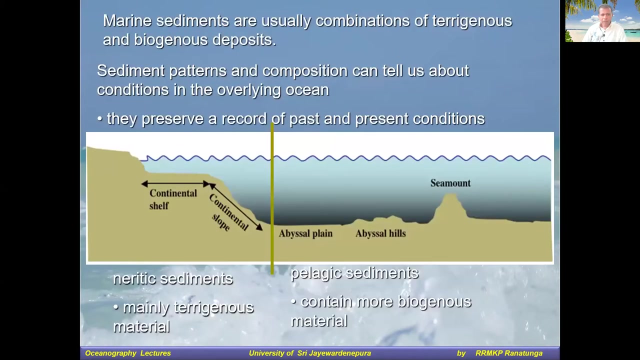 So I did this kind of exploration. In particular, I used these minerals when they were not there. If the amount of this is too much, then this is a big problem, Then the cost is too high, We don't know. Anyway, that's a little bit about the marine sediments. 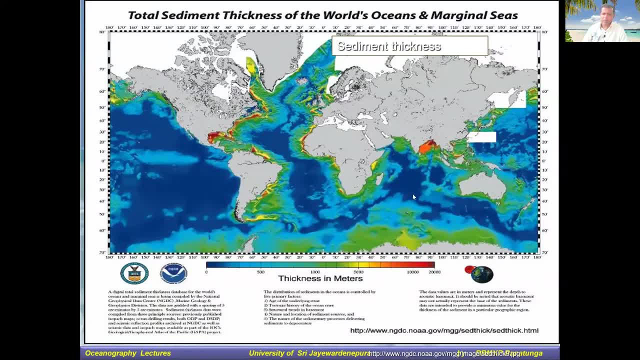 In the world map you can see where these sediments are deposited and how much. In this world map it shows the thickness of the marine sediments. The color in the sediments It indicates the thickness in the meters. Dark blue means less than 250 or 200. 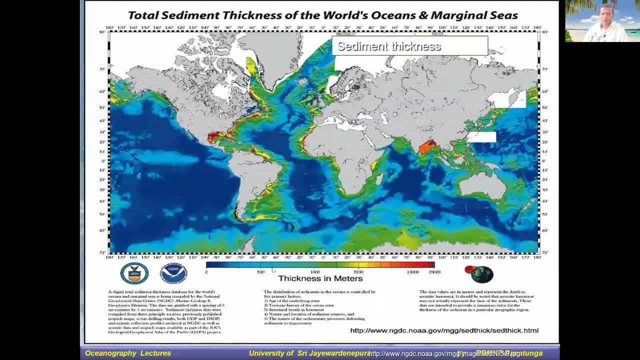 Light blue somewhere 200 to 700 or 600.. The green around 1000 to 2000 or 2050.. Yellow: 5000,. likewise, The red colors are more than 10 kilometers deep In some areas. 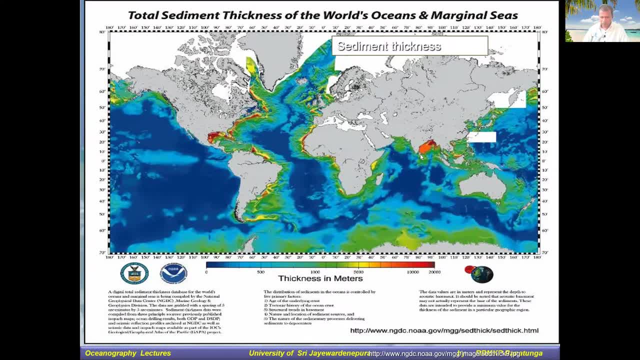 So where is Sri Lanka? It's here. Sri Lanka has a lot of deposits. Many of them have been deposited, So that's where we might have some future prospects. This is the place to look at. We don't know what is in this sediment. 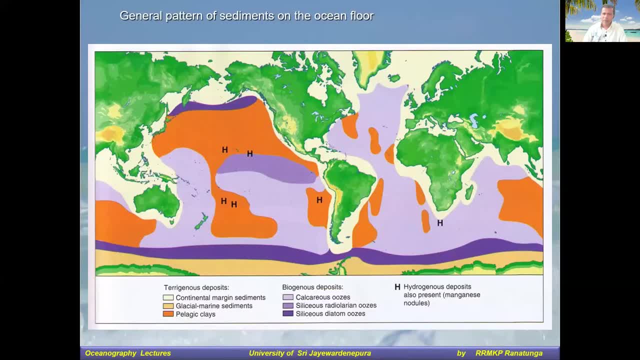 There can be a lot of very valuable minerals And this is another world map showing the world map with different types of sediments. I mean this is very rough. This is a map based on the available information. The yellow color means continental margin sediments, which means basically the terigenous sediments. 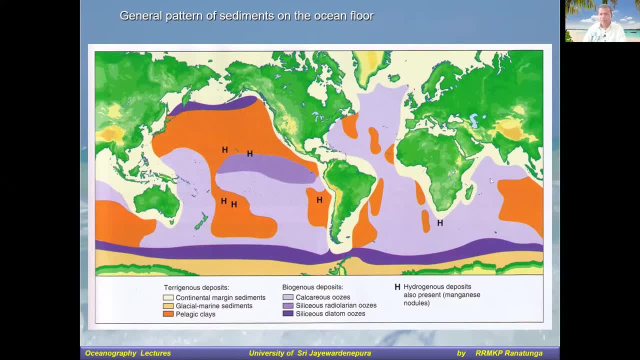 And purple is calcareous oozes. So that's basically what is around Sri Lanka: No indication of any hydrogen sediments. That's where you have a lot of hydrogen sediments. But these maps, as I mentioned, these are very basic maps without much exploration. 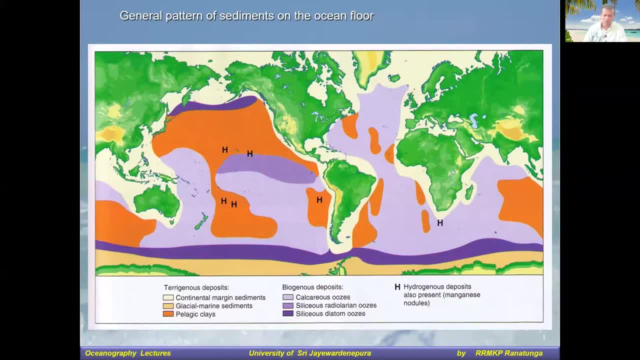 Actually we don't know anything about our ocean. There have been some experiments, but not really deep waters. We haven't done any deep water explorations looking for anything other than the oil. But we'll talk a little bit under the marine resources towards the end. 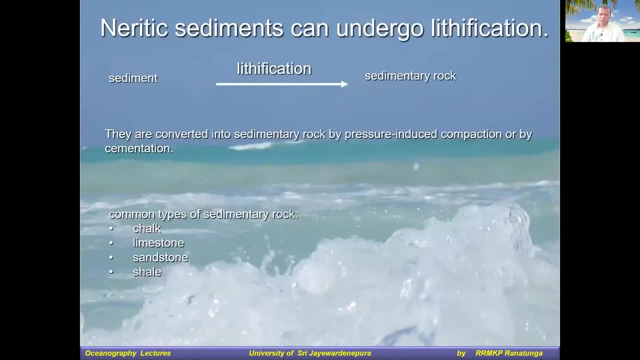 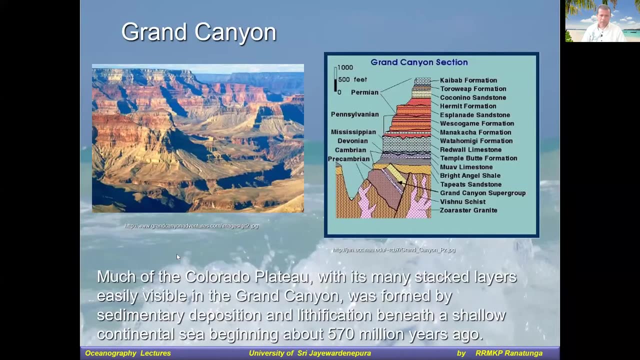 So that's basically the marine sediments, And in this image you see the Grand Canyon in Colorado in the US. This is the Grand Canyon. This is the Grand Canyon. This is the deposit. This is the terigenous sediment. These are the terigenous sediments. 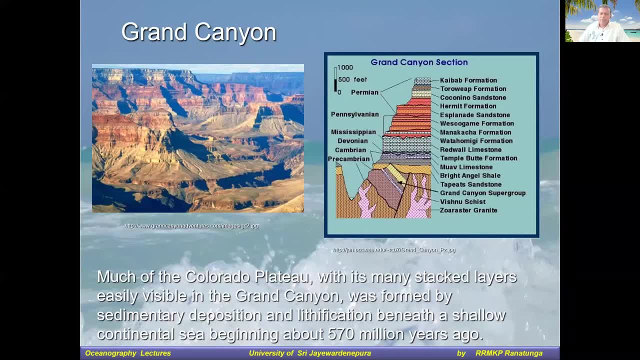 Sedimentary deposits. Now, this is Godavima, This is the ocean, But this is. I'm not saying that the ocean was in this area at that time. This is a little far from Godavima. The ocean was there in the past. 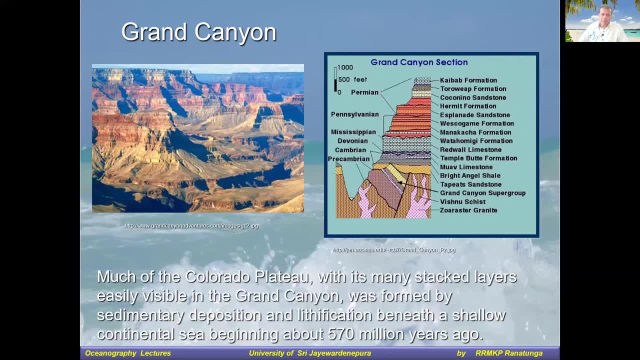 So these are sedimentary deposits that were in the ocean. Now let's talk about what these canyons are. This is the continental shelf. Now, in the past, this continental shelf is what we see here- The ocean receded. 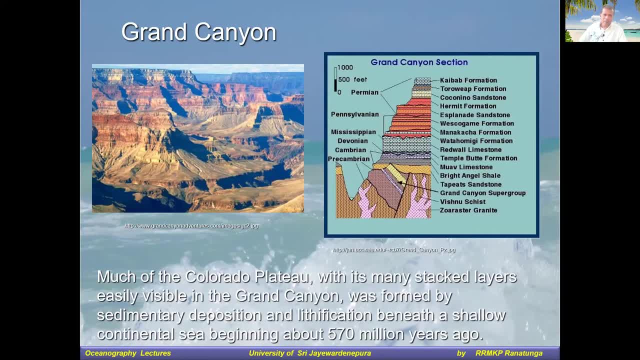 The ocean went back, But there was a continental shelf. Now we can see Godavima. Now some of you may have seen it. These are deep valleys, Valleys that have been around for a long time. This is a very important tourist destination again. 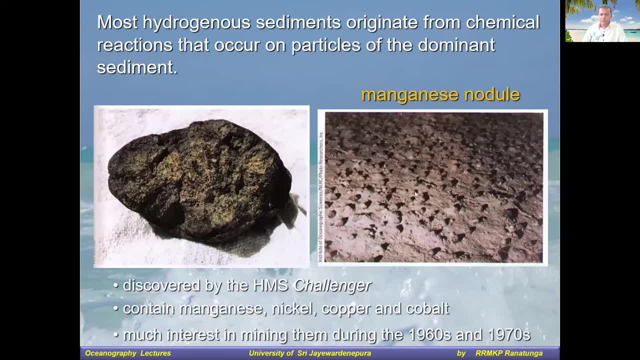 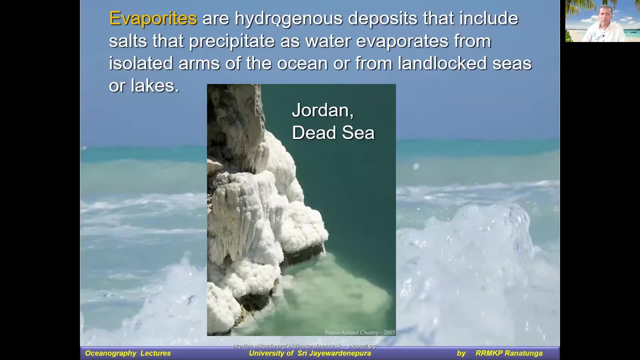 And this is where you can see the actual images of manganese nodules deposited in the ocean bottom, And this is the, And this is the Jordan Sea, as I mentioned before, The evaporites or the hydrogenous sediment deposits. This is the natural salt. 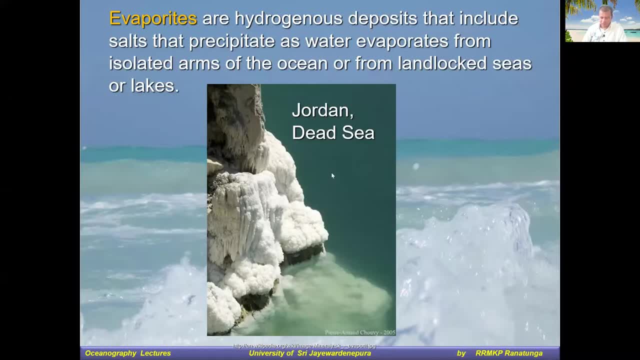 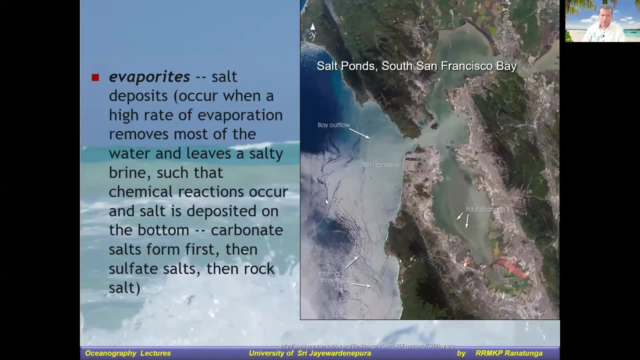 The natural salt deposited in the Jordan Sea right. I was now to Lanka. what in AMEA? See salt Right. Like what I. This is San Francisco Bay. You will see the, The evaporites, deposited in here, All right. 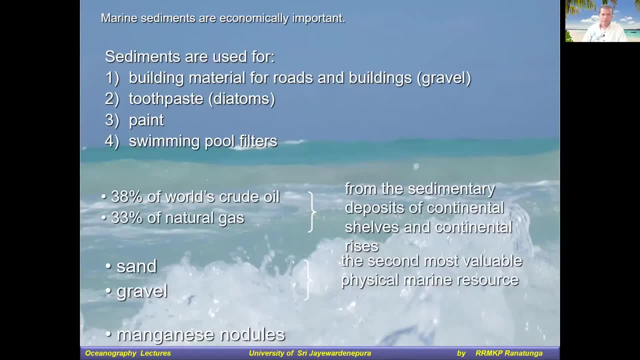 So that's about the marine sediments. Other than that, that's all about the marine sediments. I hope you got some idea. My thing was a bit difficult, Of course, since you are listening to this for the first time. 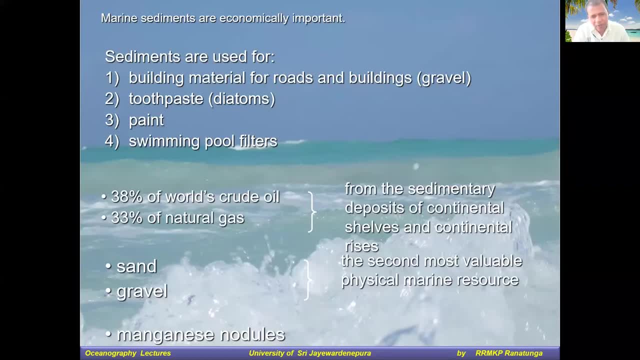 And geology is not most of us favorite subject, But anyway, yeah, You just need to have a very good, very basic knowledge about the types of marine sediments, Especially the uses and how they can be used, And that's all for the day. 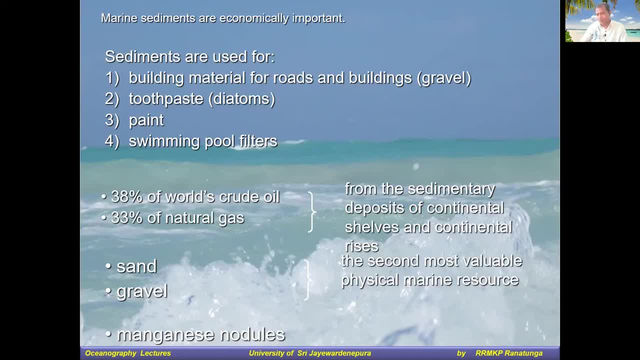 And then in the next week we will start with the branding, A brand new topic, Especially one of I hope you will enjoy, Because that is where we'll talk about the movement of the ocean, Especially the waves, tides, the currents. 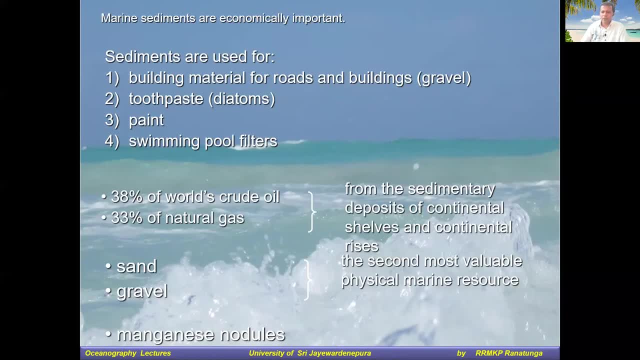 And that is very much not like the geology. We haven't seen anything But the waves, currents, something that we are all familiar with, And we will see how these waves are formed And how the tides are formed, And what are the currents and waves and tides.